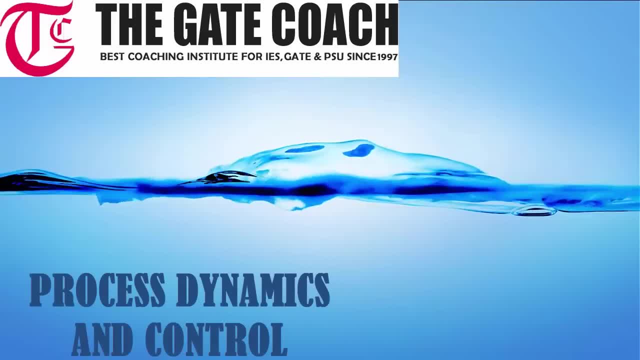 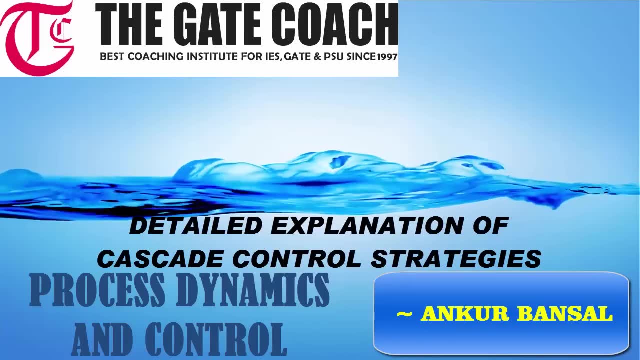 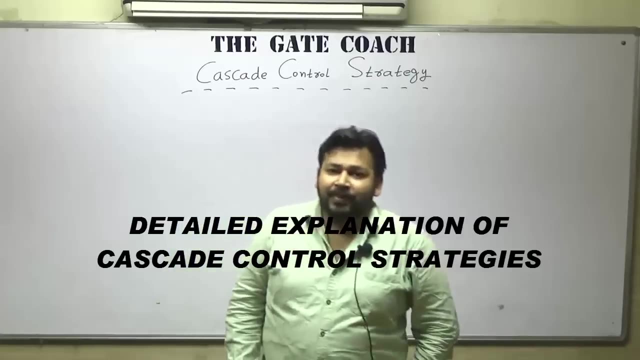 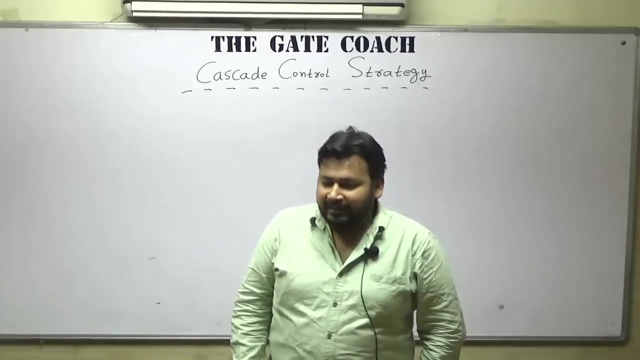 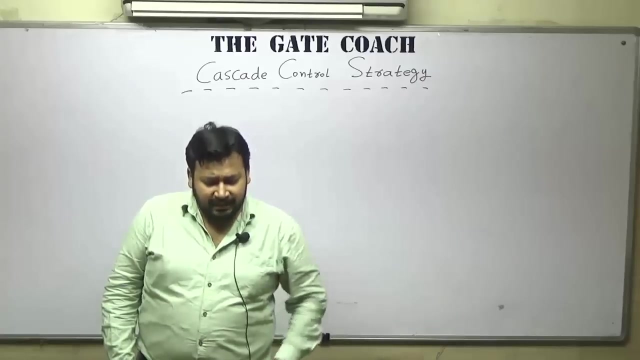 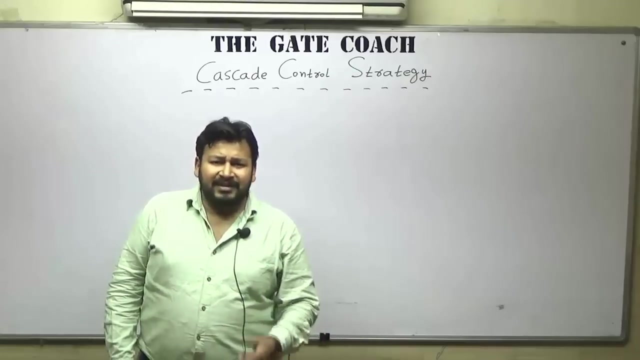 Good morning friends. today we will discuss about one of the very, very, very important topic of the chemical process control, and that topic is none other than cascade control strategy. So today we will detail in detail. we discuss about this complete strategy and before watching this video, I will suggest that watch my previous video on the two strategies, that is, feed backward. 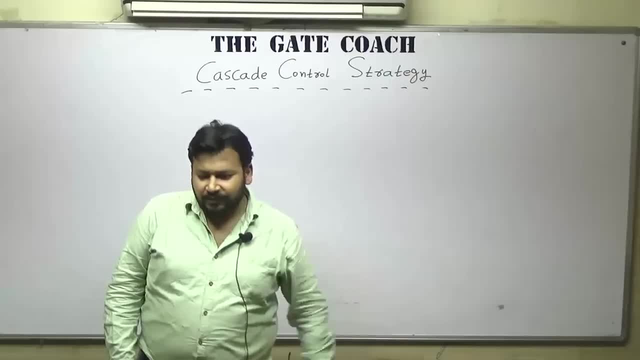 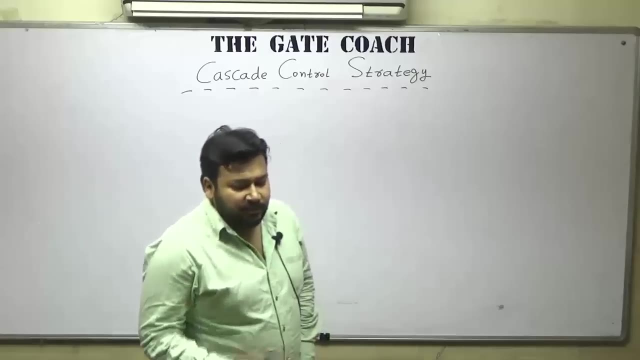 and the feed forward. So must watch that video and after watching that, when you have the correct knowledge of the feed backward and the feed forward, then it will be very easier to understand about the cascade control strategy. So before studying into cascade control strategy, first of all we need to realize that. why cascade? 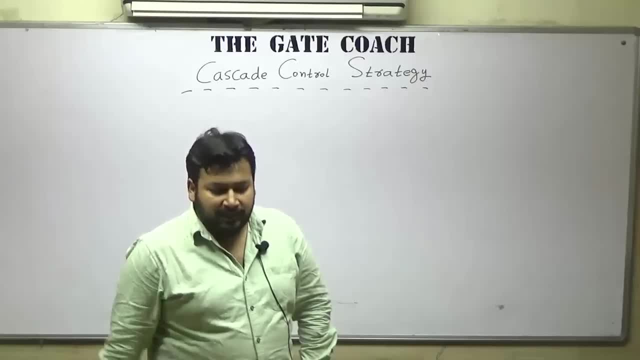 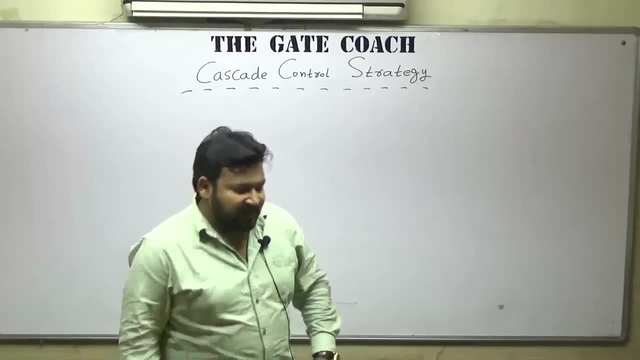 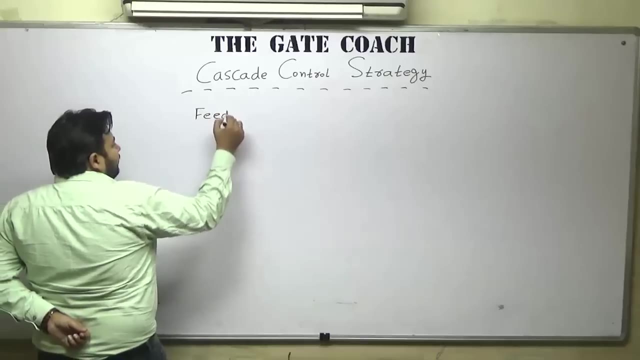 control is required. If we have the feed backward and the feed forward strategies, then what is the need of the cascade strategy? So, first of all, we will understand that and to understand that, we will refer feed backward control strategy, As I discussed about this in detail in the 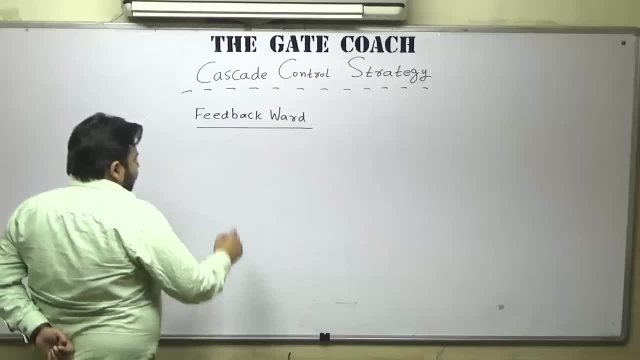 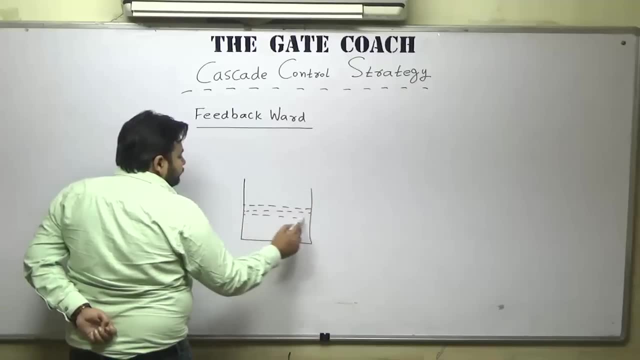 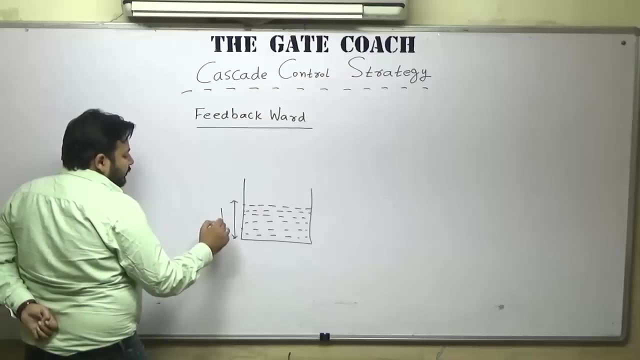 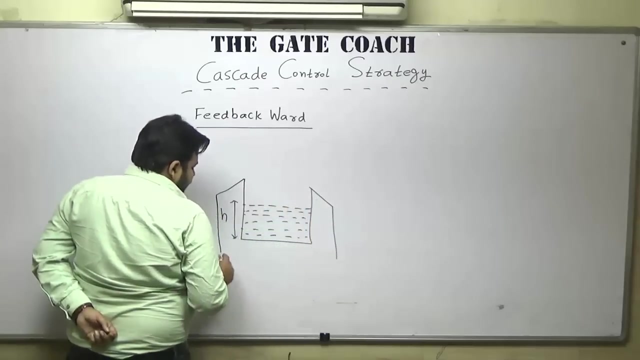 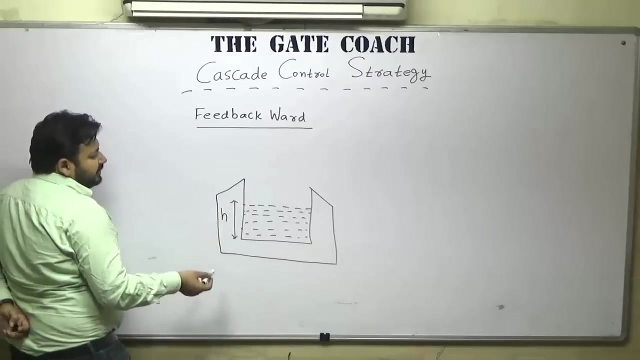 my last video feed backward control strategy. So on the feed backward control strategy. there is a tank, There is a tank and this tank contains liquid and this liquid is having a height H. Now in this tank there is some reaction going on And there is a jacket That can be cooling jacket, that can be a heating jacket, that 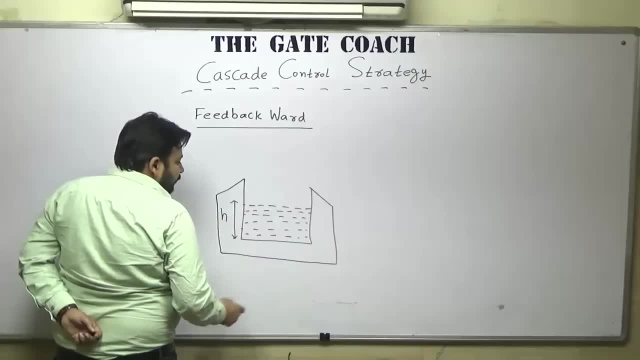 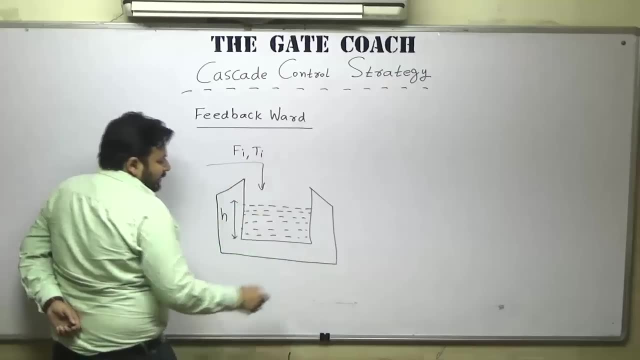 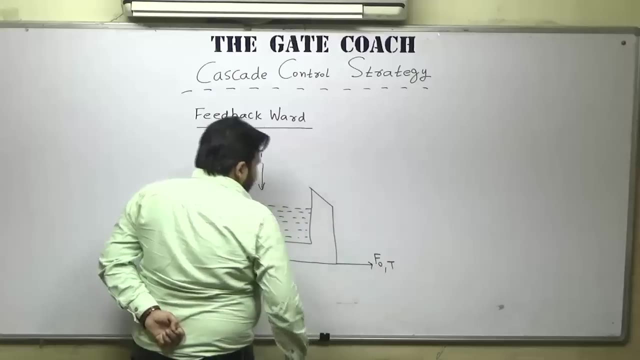 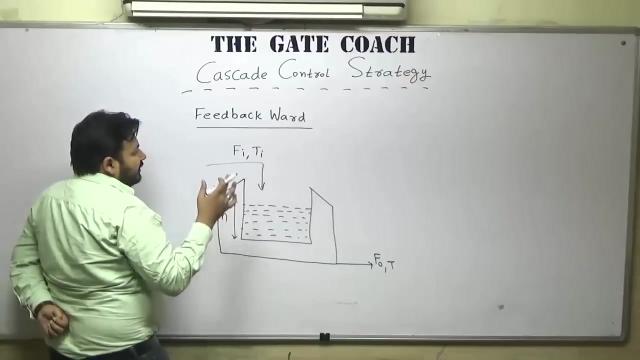 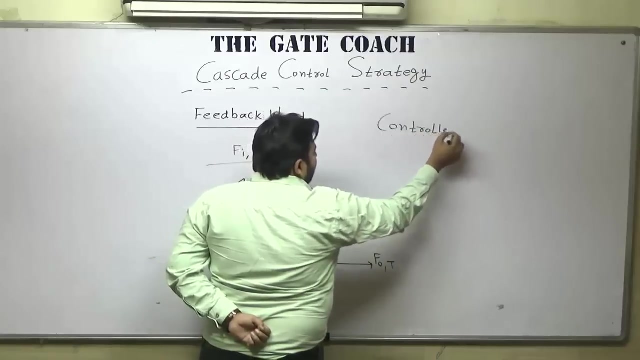 depends. So there is some inlet with a flow rate Fi and with a temperature Ti And there is some outlet with a flow rate F0 and the temperature T And the main controlled variable. as we discussed in the last class about the, we should have the knowledge of controlled variable. now, what is controlled variable? 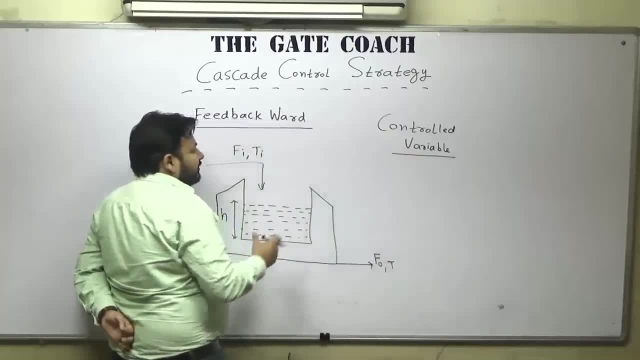 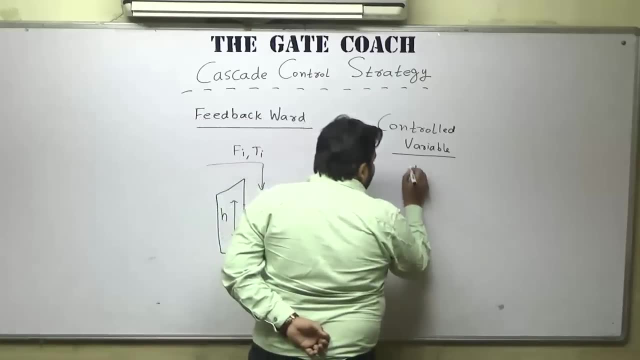 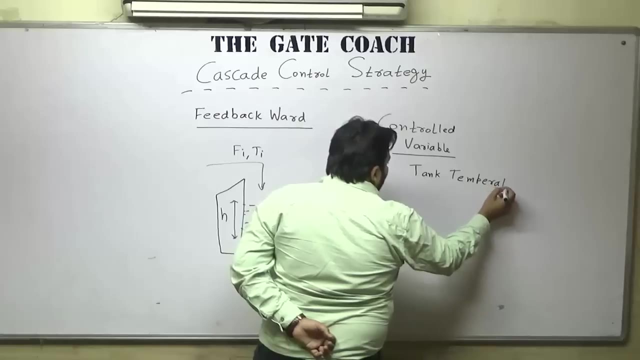 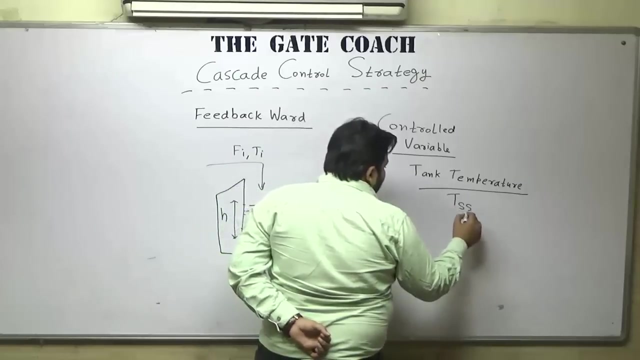 controlled variable is the purpose of the system, is the main objective of the system. and the main objective of the system here is the tank temperature, tank temperature- that is the main objective of the system. and let us say there is a steady state value of the temperature. so our main objective is to maintain this tss value in the tank. 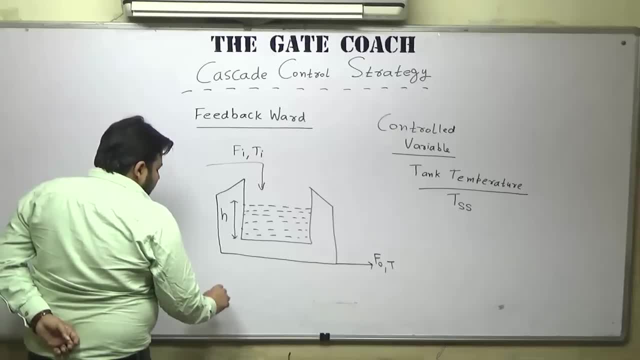 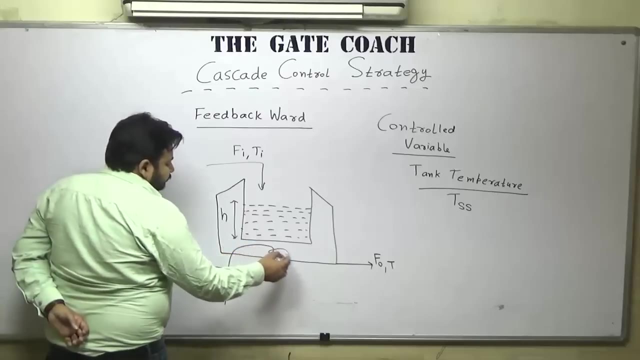 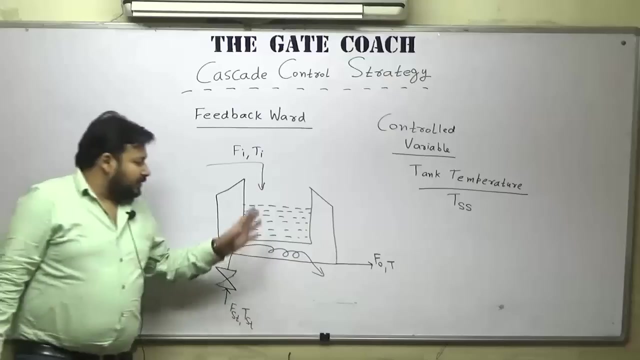 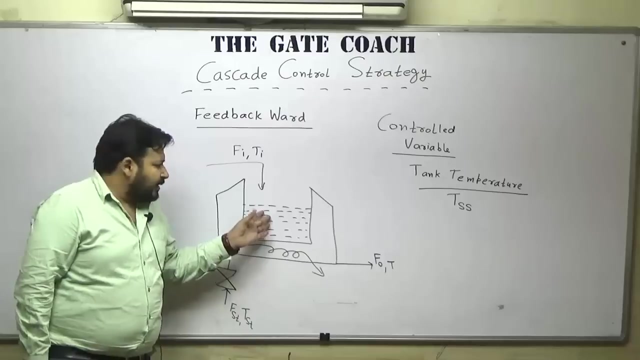 now to maintain that there is some continuous supply of- or you can say- steam. there is a continuous supply of steam is there in this jacket. so that is a simpler system. now let us understand the system. there is a, there is a reactor. in this reactor, some reaction is going on. there is an inlet. 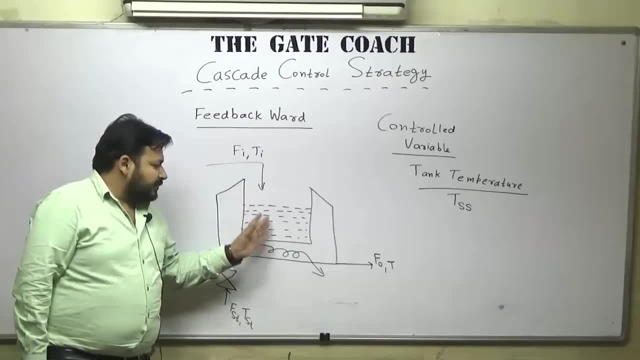 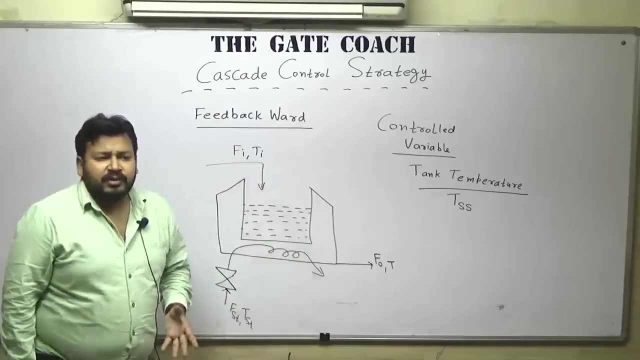 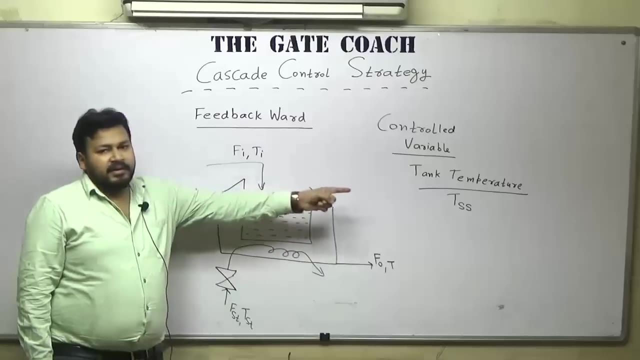 there is an outlet and to maintain a desired amount of temperature in the reactor, we are passing a steam through it. now, initially assume the complete system is at a steady state value, so the temperature of the tank is tss. now, if there is any change in the flow rate, 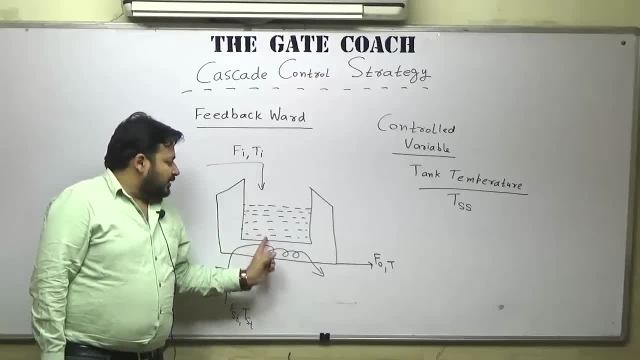 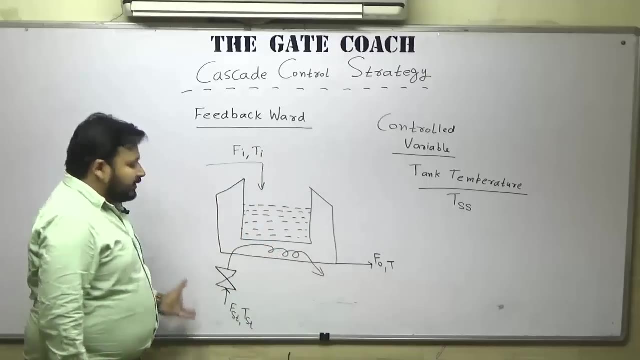 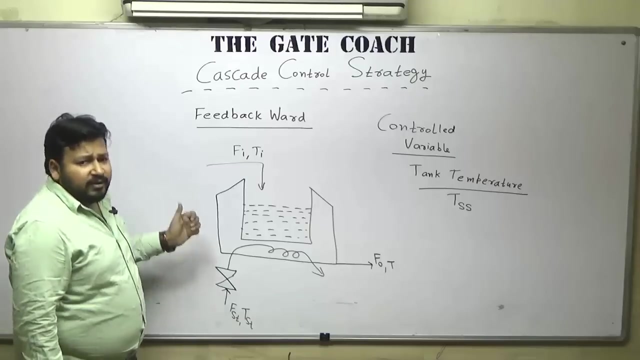 let's say, the flow rate increases, the level will increase, and now the more level, that means more amount of liquid will need more steam to maintain the temperature, and but there is no controller here so no one knows it. so we cannot. we cannot open the wall, we cannot close the wall. so what will happen if fi changes? 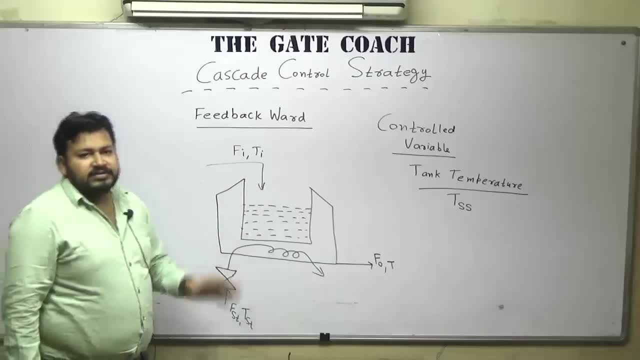 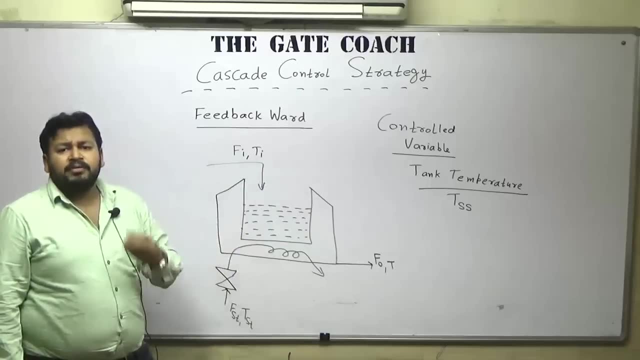 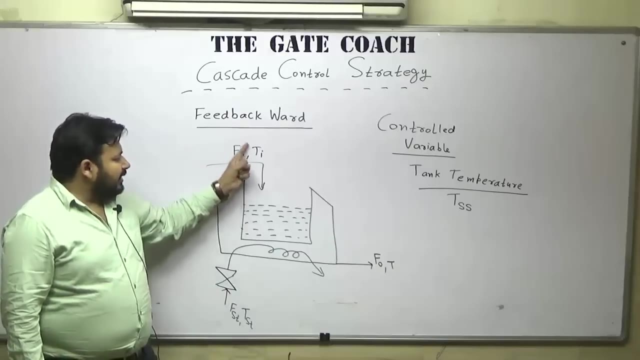 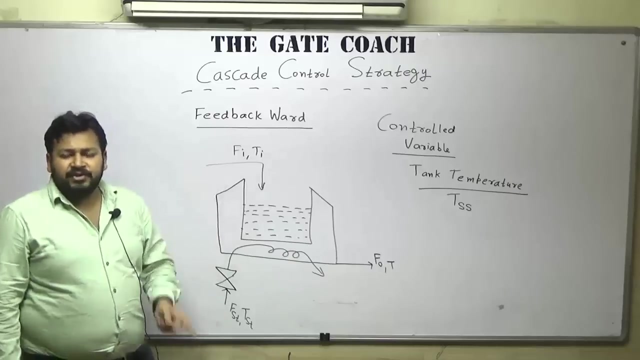 the temperature of the tank will change, the steady state will disturb. so that's why to control, we need a control system here, take care. so that is the answer of why: control system: to suppress the effect of external disturbance, this is the external disturbance. to suppress the effect of external disturbance, we need a control system. so what will i do here? 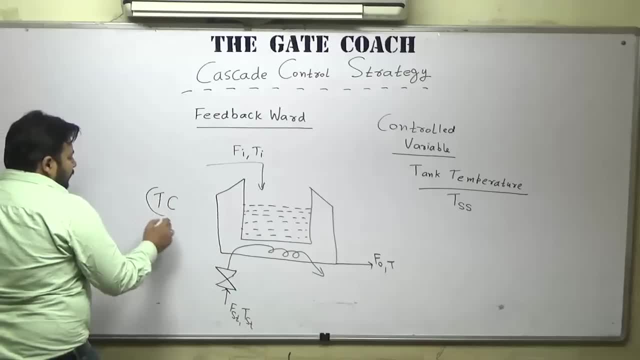 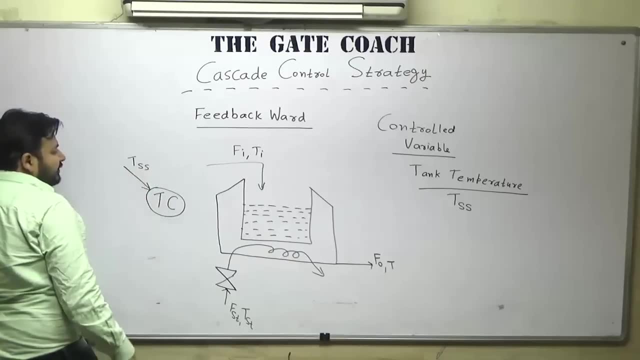 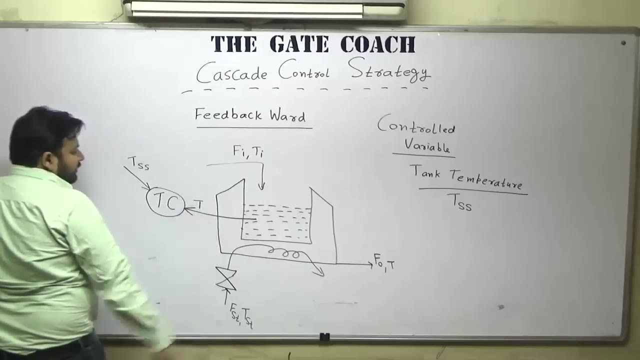 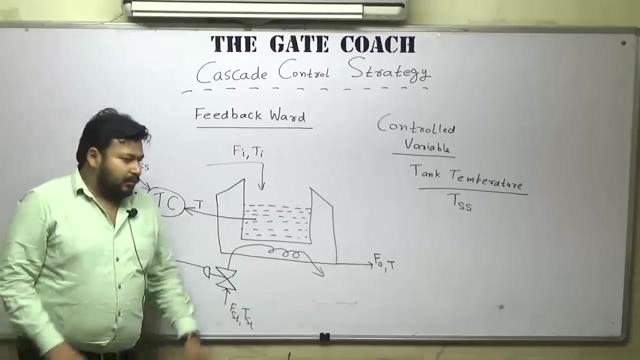 let us say there is a temperature controller and to this temperature controller i am inputting a steady state value of the temperature, that is tss. simultaneously, i am measuring the tank temperature, that is, let's say, t, and on the basis of the difference the temperature controller walk and open and closes the wall. now look at the same scenario. 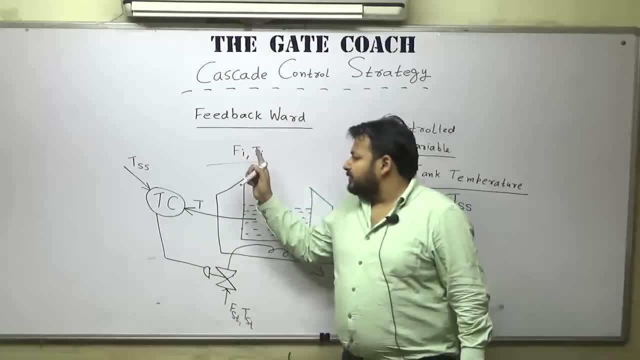 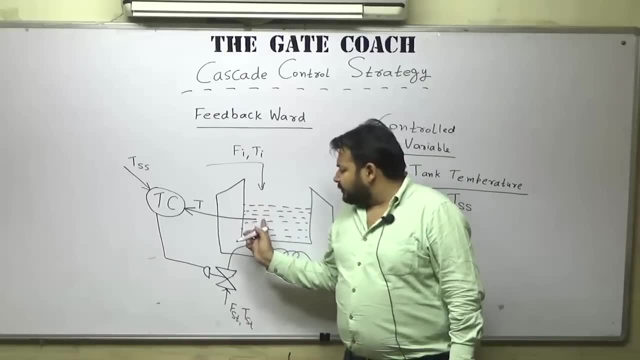 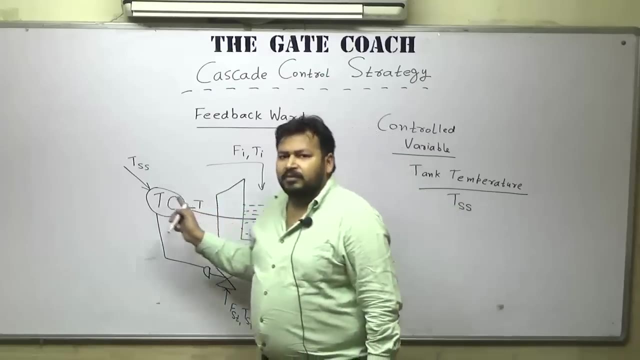 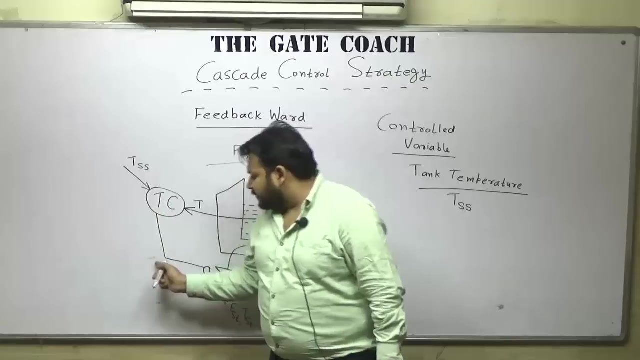 again, if the flow rate is changed, this changed flow rate will change the temperature of the Hawaiiiac, so we can see temperature of the reactor is going. have registered the temperature of the reactor and as the temperature of the reactor changes, this value will change. and as this value will change, this minus this, there will be a non zero error. 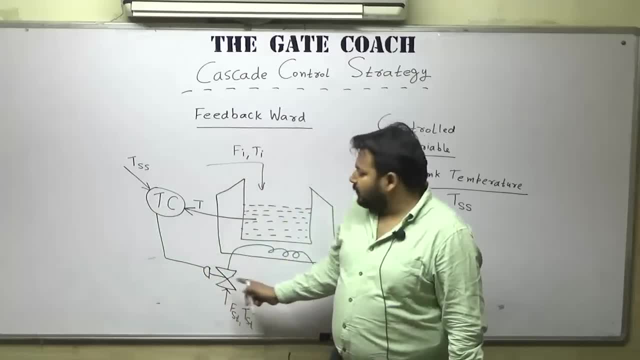 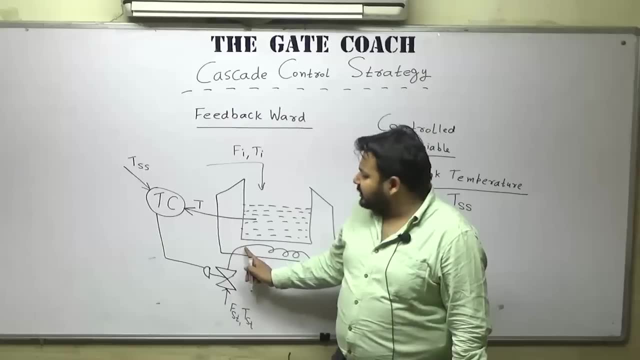 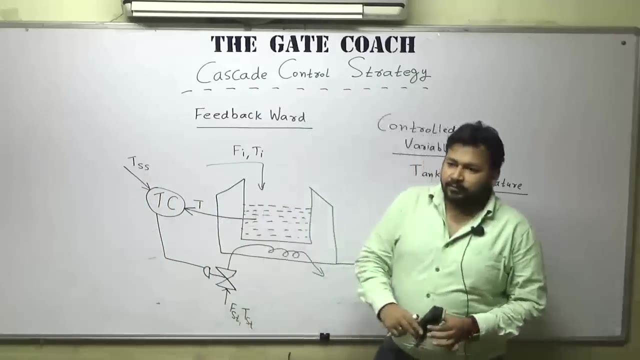 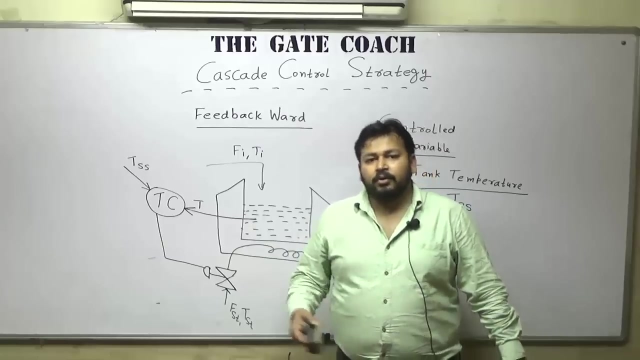 and to minimize that non zero error, controller will take the control action and changes the opening of the wall and ultimately, as the vol opening changes change, the temperature of the reactor will change till we get the desired value. so by the help of feedback control strategy, by the help of a control system, we can maintain the steady state of the 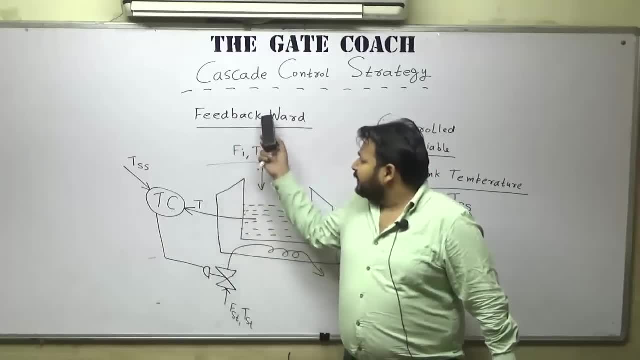 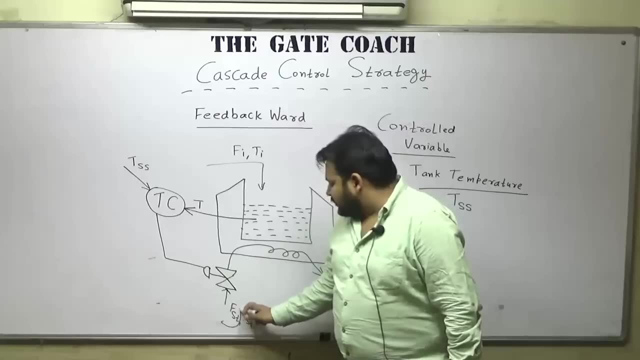 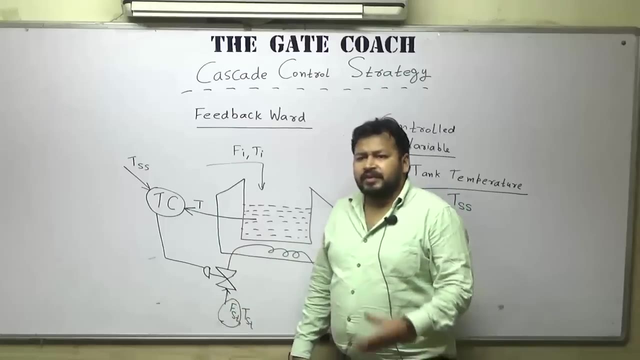 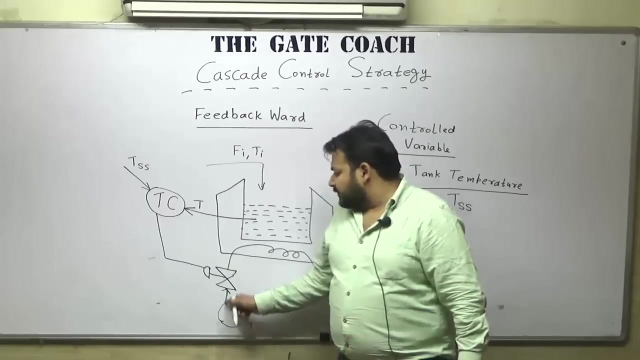 system that is feed backward. now understand if there is any change in the steam flow rate. let's say initially the steam is some X amount per hour coming in and after some point of time there is a disturbance in it, but steam flow rate increases. or may be steam flow rate decreases because this is an input variable. or you can say this is: 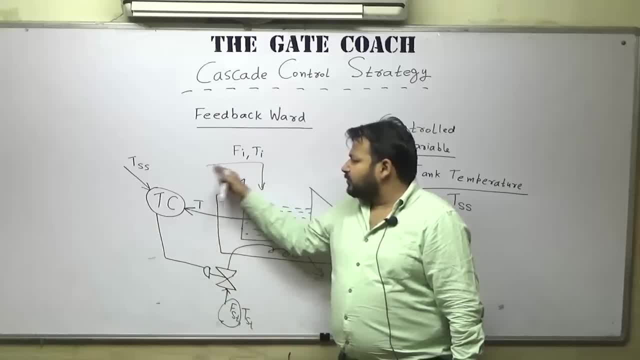 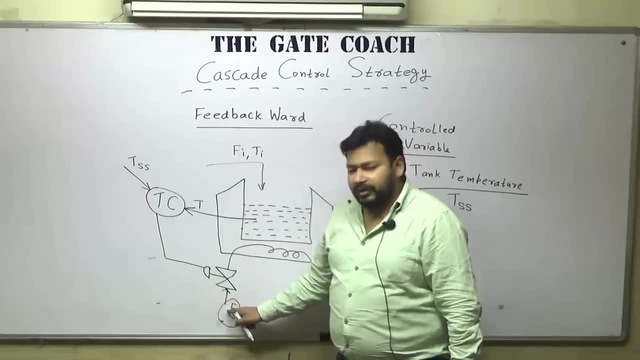 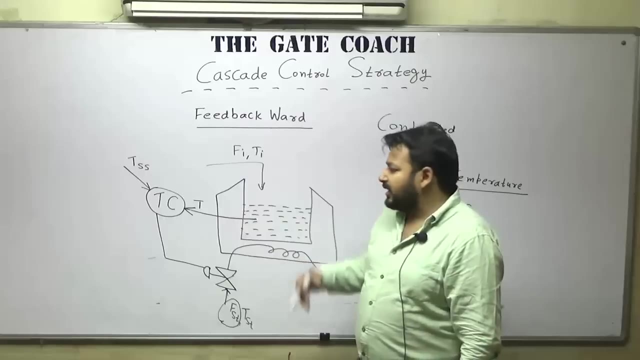 a disturbance variable like this can change on it's own. this also can change on it's own. so if there is a any change in the steam flow rate, what will happen? the temperature of the jacket will change and as the temperature of the jacket changes, there will be a change in the tank temperature again. 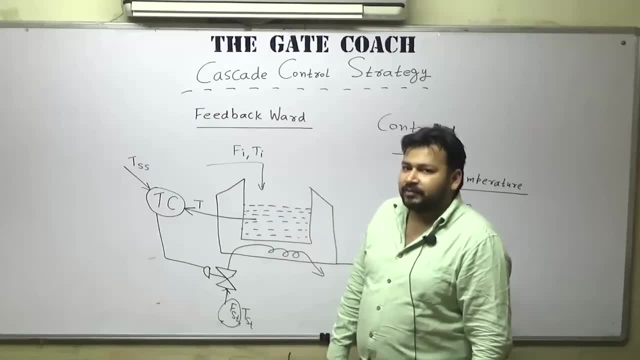 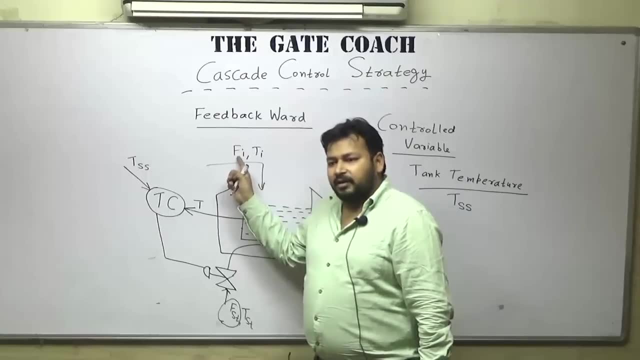 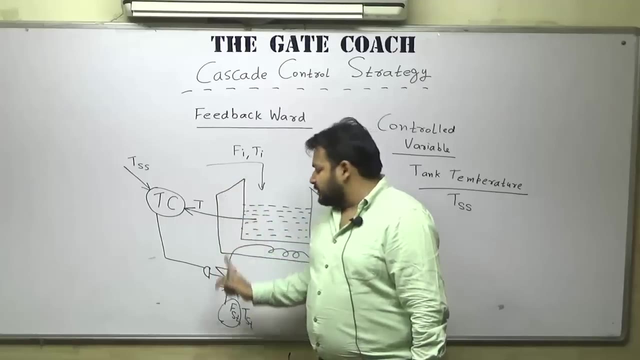 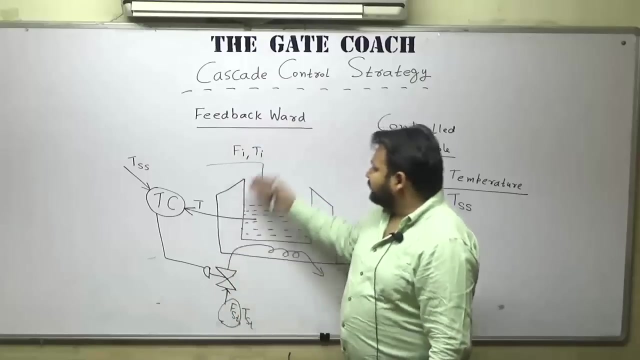 that means in this diagram, in this system, the number of disturbance is not only the tank temperature can change, but this also can change. you can study this in terms of flow rate or you can study this in terms of temperature also, because of the inlet is having a different. 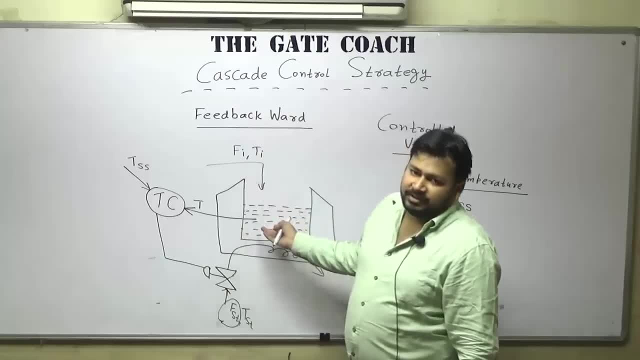 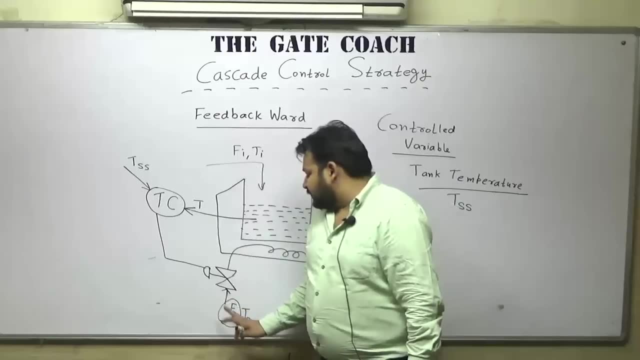 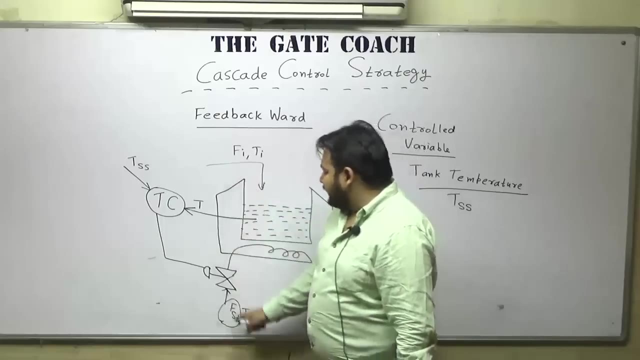 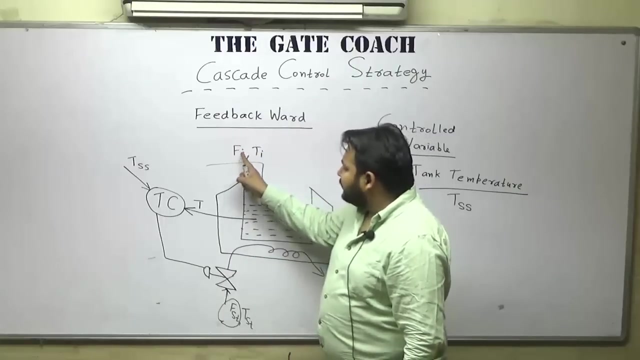 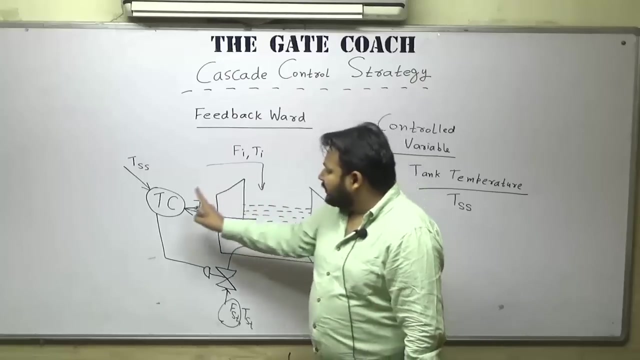 temperature. it may affect the tank temperature but for the time being we are focusing on the flow rate values. so as electricity changes, then also the tank temperature will. both are the disturbance, but the nature of both the disturbances are different. how carefully? as fi changes, it will affect the tank temperature directly and as there is any change, controller or sensor will sense that. 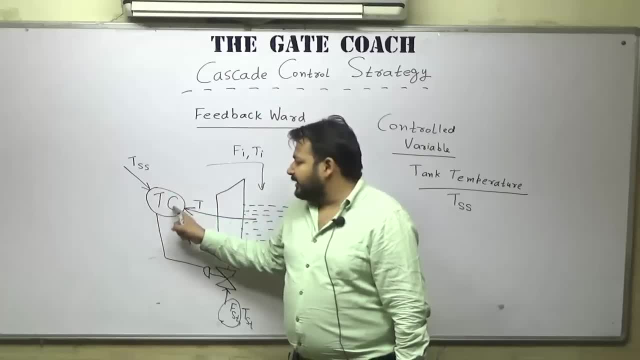 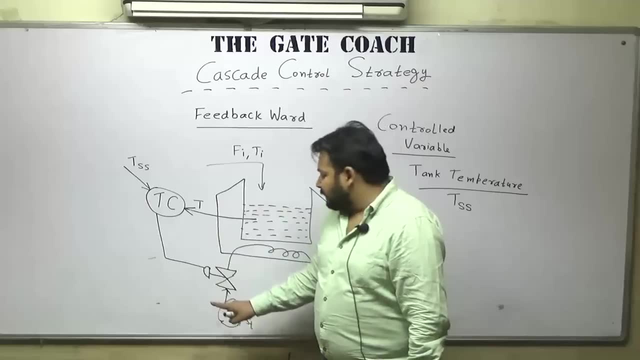 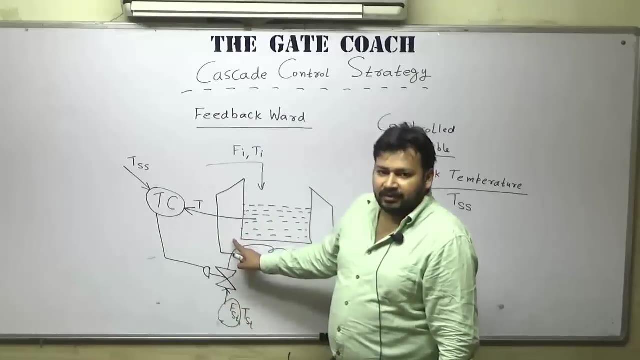 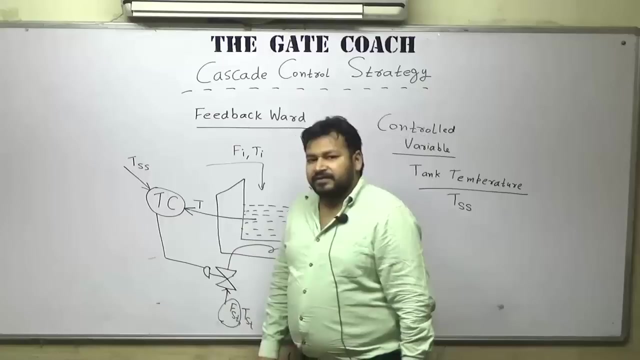 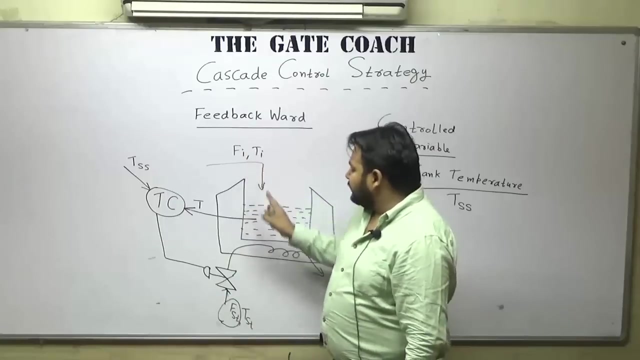 change immediately and control action immediately. but if there is any change in the steam flow rate it will not change the tank temperature directly. first of all it will change the jacket temperature and then it will change the tank temperature. that means any change in the fst cannot be sensed by the sensor directly. but if there is any change in the fi, then this: 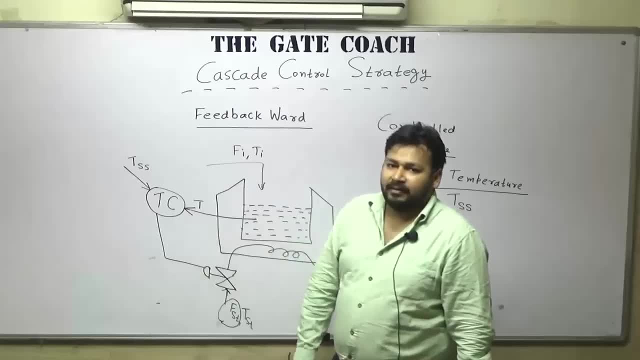 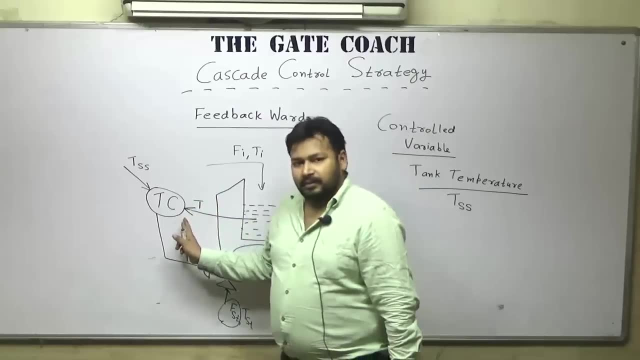 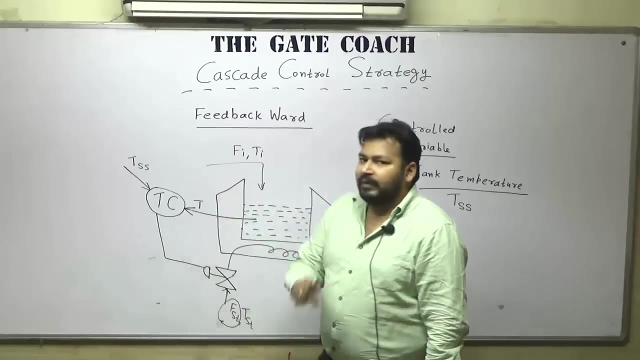 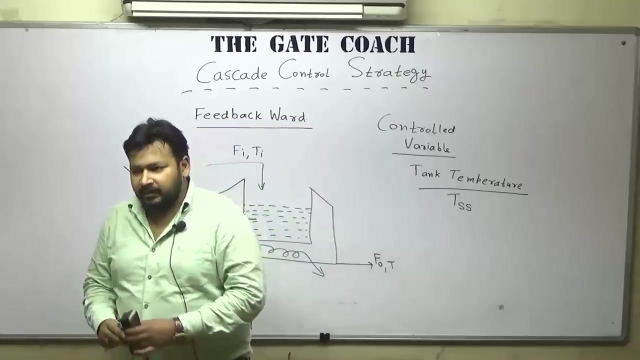 stage can be sensed by the center directly. that means our control system and our control strategy is affecting to suppress the effect of fi but is less effective to suppress the effect of fst. that means this control strategy is not effective for all the disturbance is effective for some of. 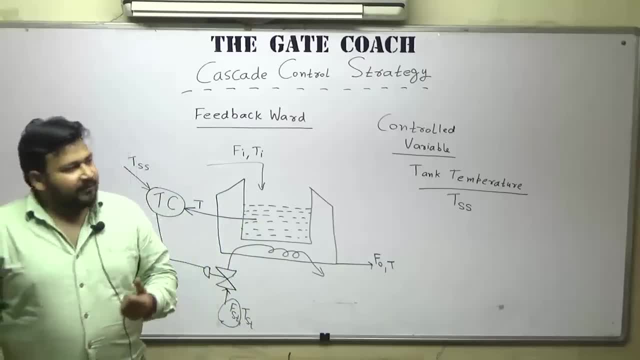 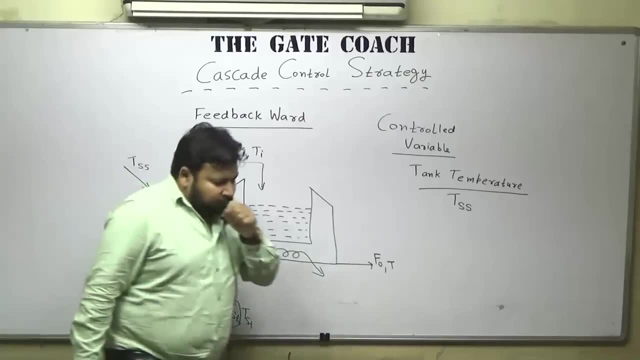 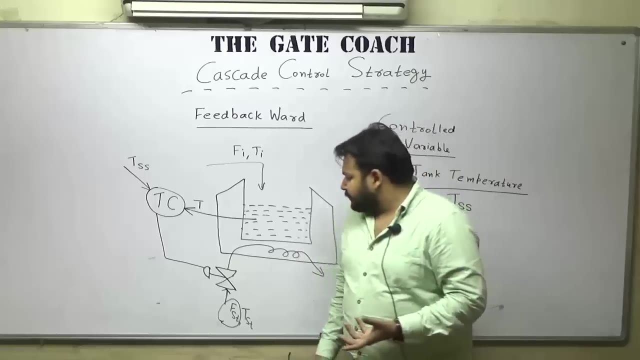 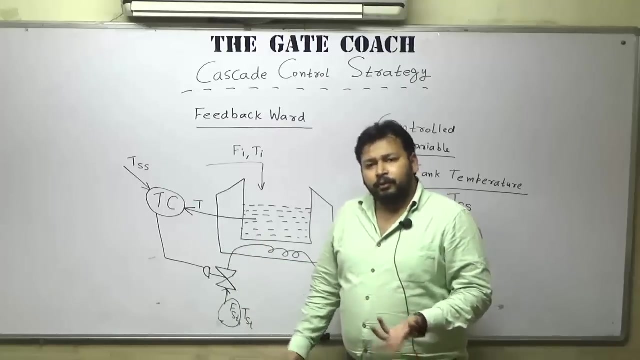 the disturbance and in this diagram it is effective for the fi but it is less effective for the fst. now, if we can bear this in effectiveness, that means with respect to fst the change is not direct. if we can bear it, then it's okay, no problem, this strategy is the best. but if this change is 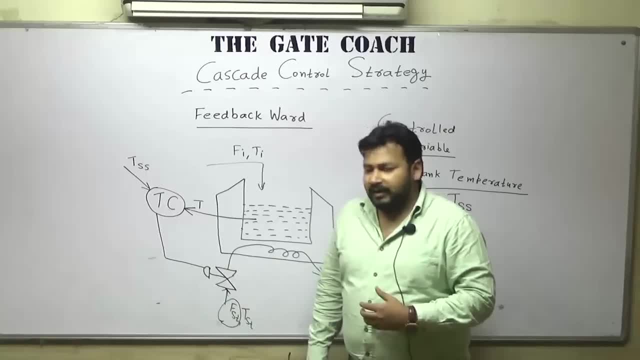 unbearable. that means if we want our control strategy to be effective for the fi as well as for the fst- both- then we need to change it. so it depends upon the economic balance, because if we change the strategy there would be some cost involved. and what? what is the reason to? 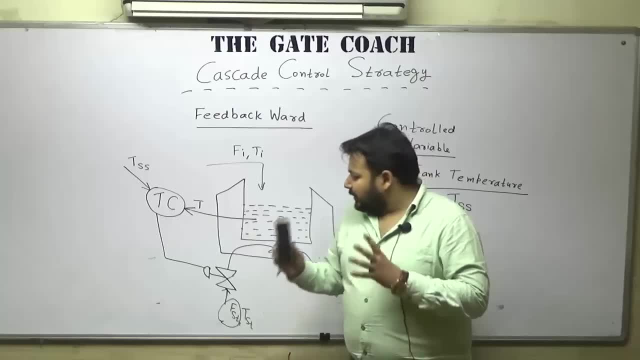 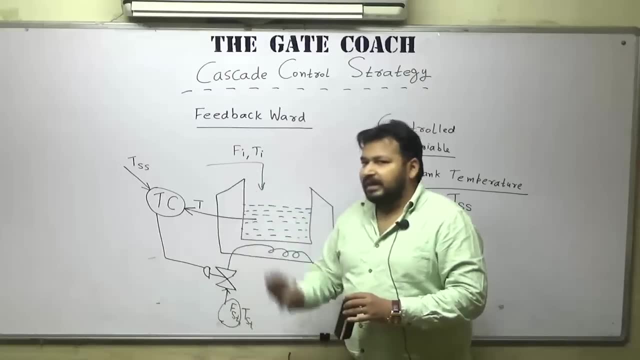 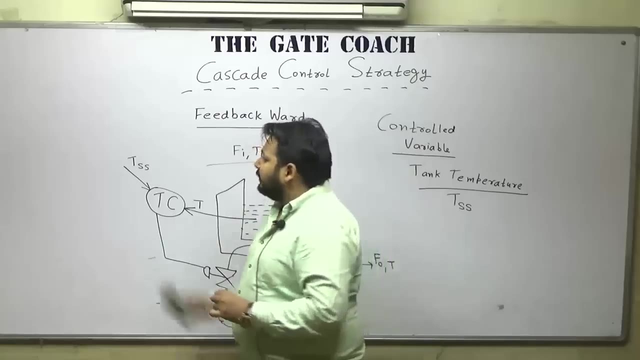 change the strategy. that also matters. so if i only, if only i want to make my system effective for both the disturbances, then i will change the feedback control strategy. and in that case, what will i do? use the cascade control strategy. so that is the answer of why cascade control? and 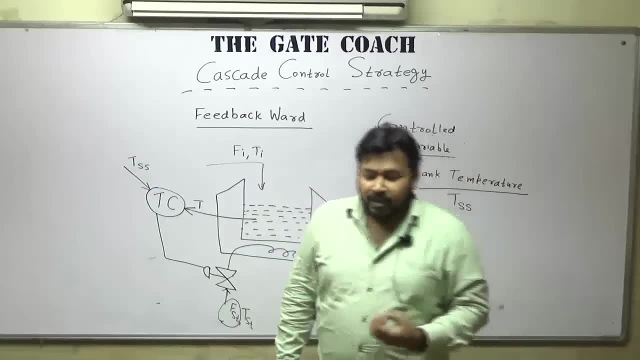 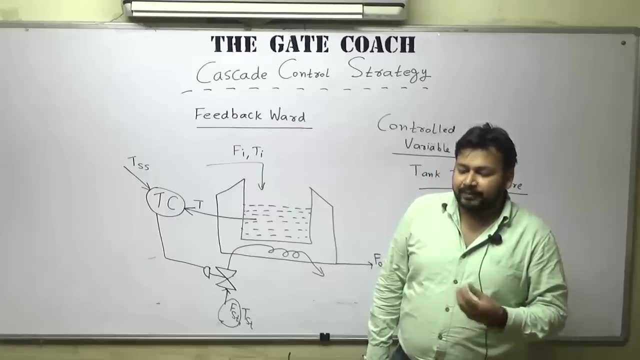 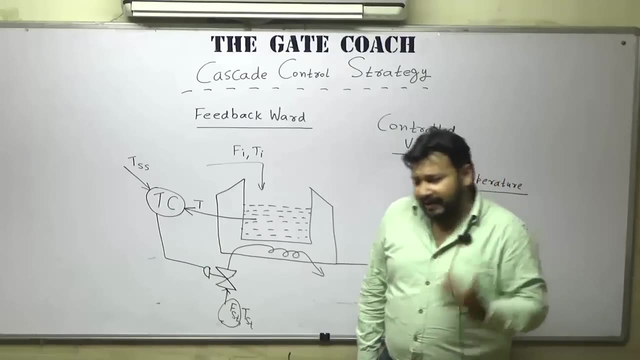 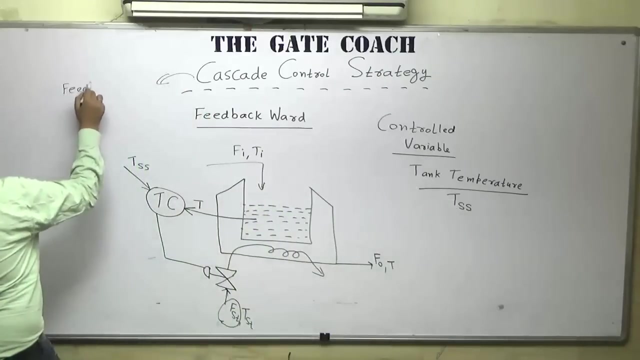 that's a very, very important question. why cascade control? because the feedback control strategy is ineffective for all kinds of disturbance, for all types of disturbance, and to make it effective we use the cascade control strategy. and cascade control is nothing but defined. it is defined as feedback in a feedback. 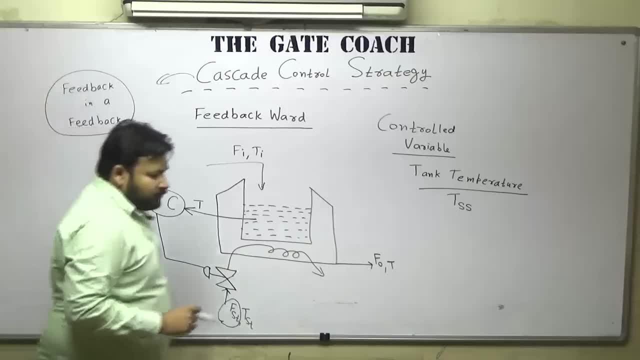 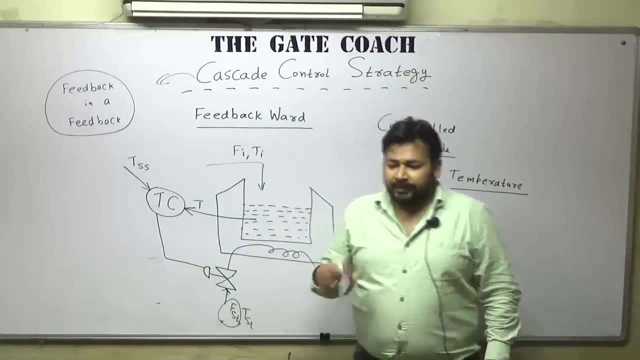 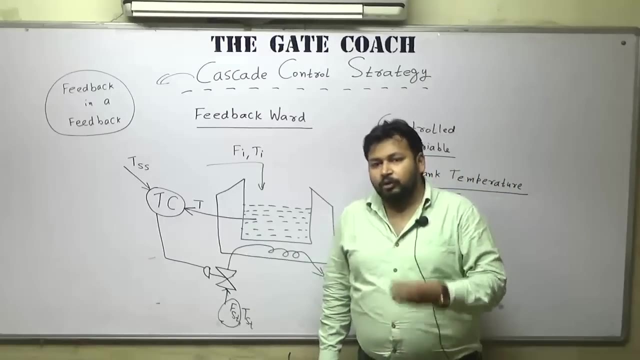 feedback in a feedback. so I will do nothing. I will just use the loop in a loop in a loop in a loop. so it depends how many loops- as let's say, the number of- are three, for which you want your loop to be effective, then you will use three. 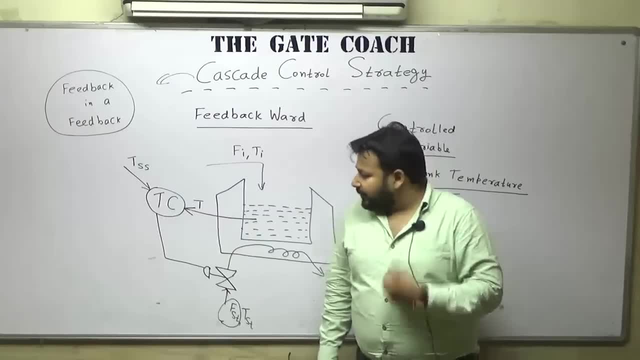 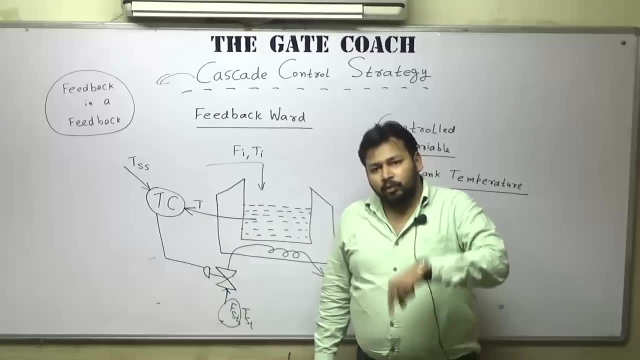 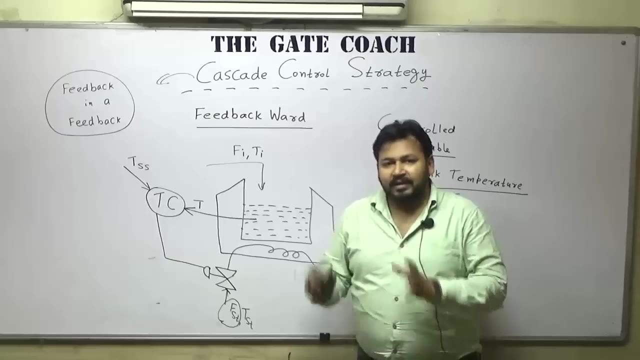 loops of the feedback loop in a loop in a loop. so it depends now here the number of disturbances are two. already one loop is there. I will add one more loop so that the control strategy becomes effective, and that is known as cascading or the cascade control strategy. so I hope I gave you the answer that why? 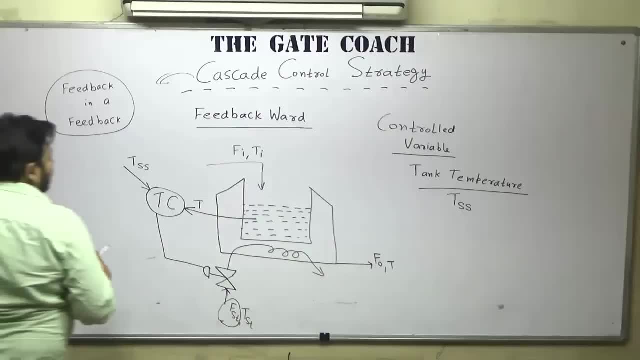 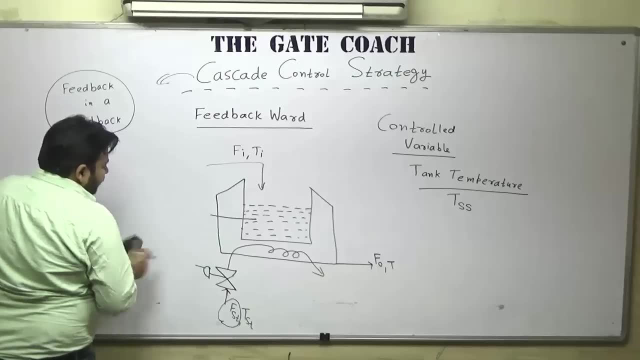 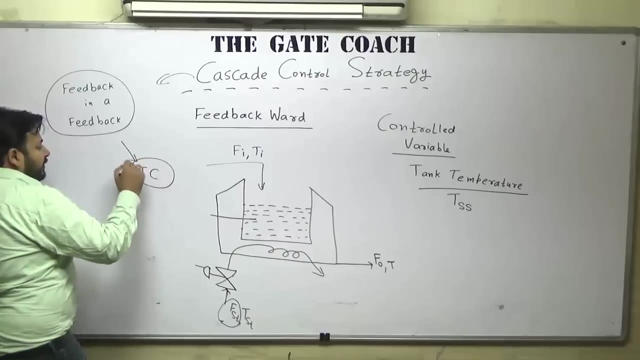 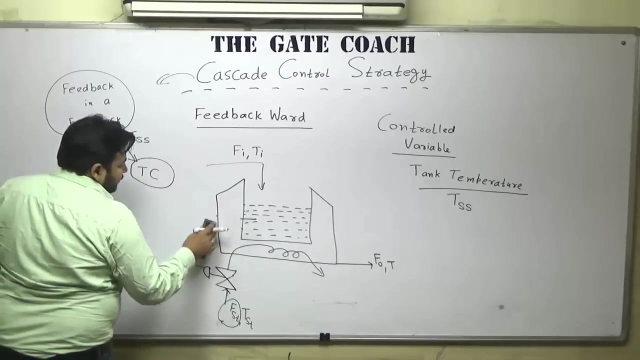 cascade control so that our feedback control strategy is effective for the both. so now, in this case, what will I do? the temperature controller will be there, there is no issue with that, there is steady state value will be again TSS and the tank measuring temperature again will be T. 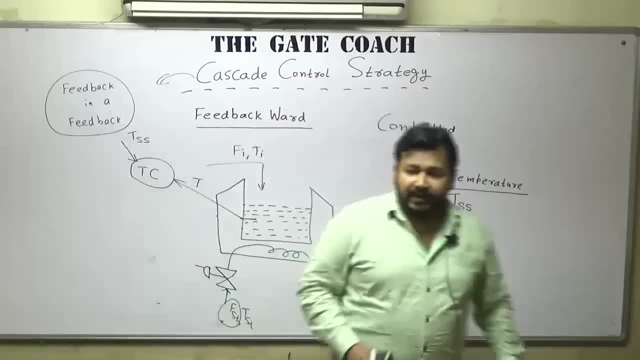 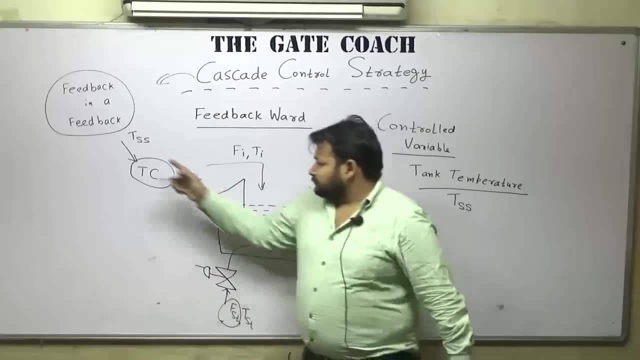 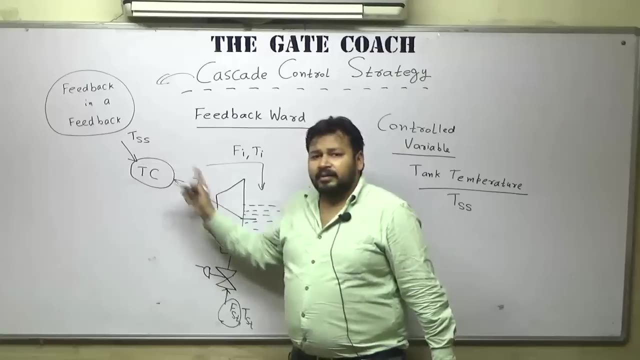 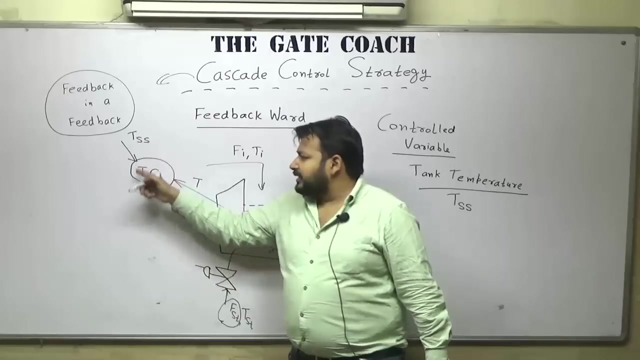 okay, to this point, it's okay, I think. now try to understand that in the last scenario, what is happening out? there is a difference between the two. whatever I want and whatever I have, there is a difference between the two. the temperature controller takes an action. now, what is this controller? what is the? 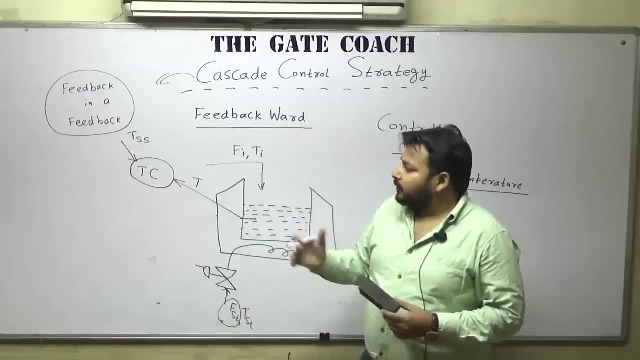 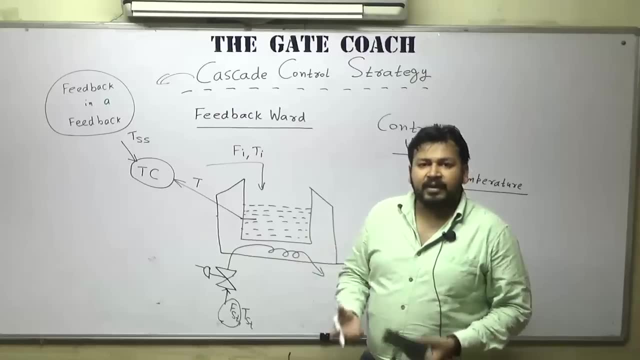 control is all about. you need to understand that a control is nothing but a set of written, some command or some program, some material balance, some mass balance. heat balance is nothing but a model that will help you to take care of the system. so temperature control here is nothing. 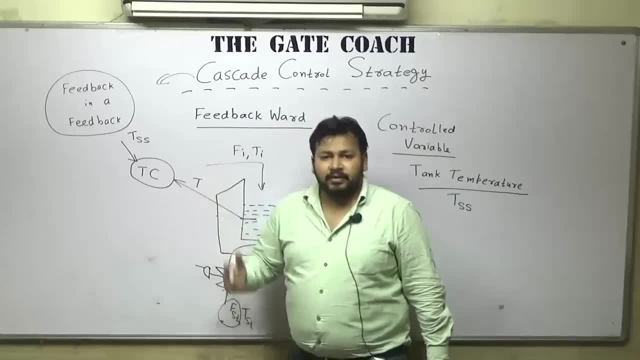 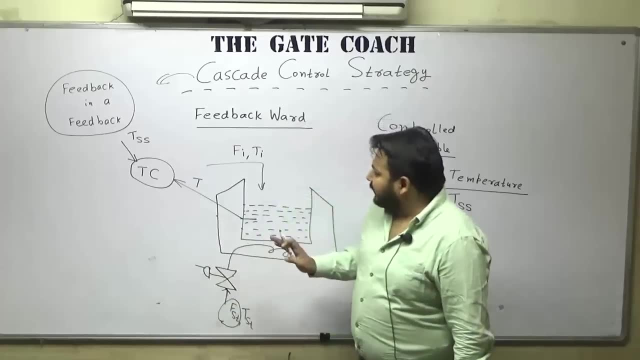 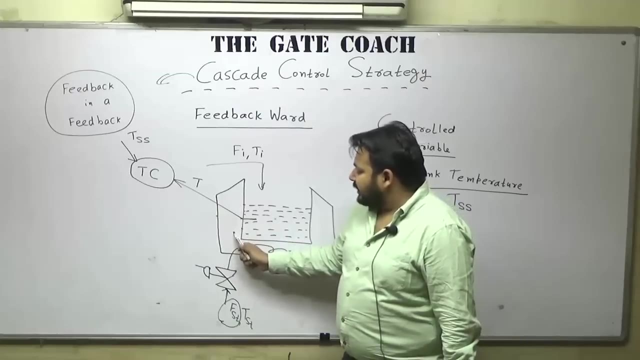 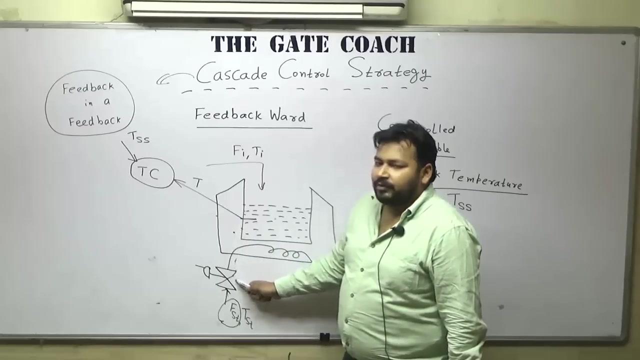 but a model. model, or you can say a set of equations in which, if we put some values, it will give us the desired value. so ultimately, this temperature depends upon the jacket temperature, and jacket temperature ultimately depends upon the steam flow rate, and steam flow rate ultimately depends upon the valve opening. so all these are interdependent. 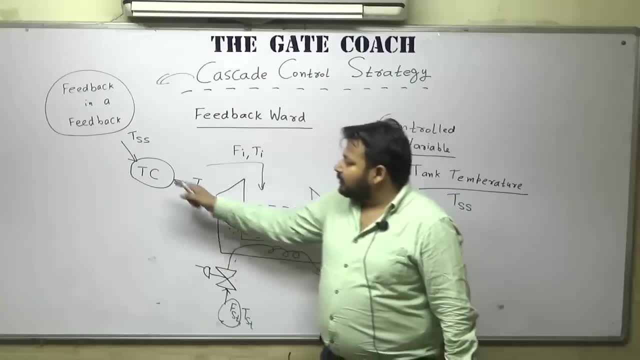 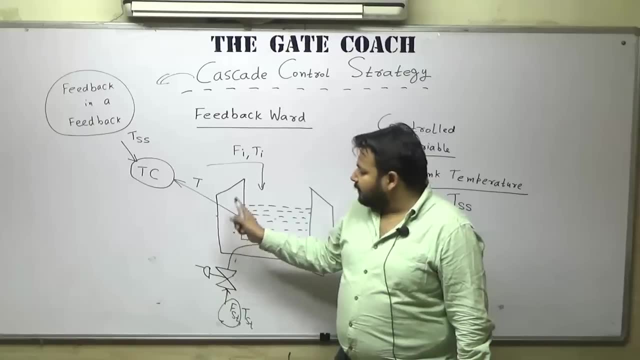 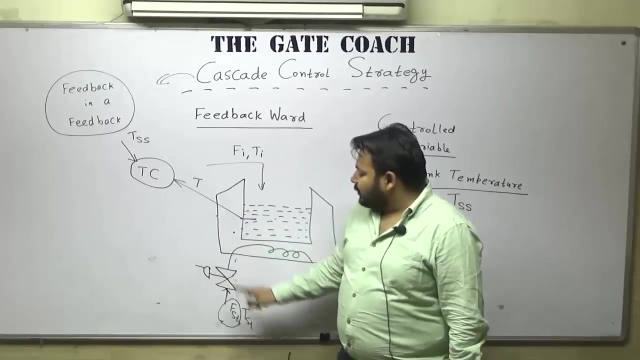 so what is the work of temperature controller? temperature controller with the help of the best possible jacket temperature. now, with the help of that value, this controller will calculate the best possible steam flow rate so that this jacket temperature can be obtained. and then, with the help of this flow rate, temperature controller will calculate what is the best. 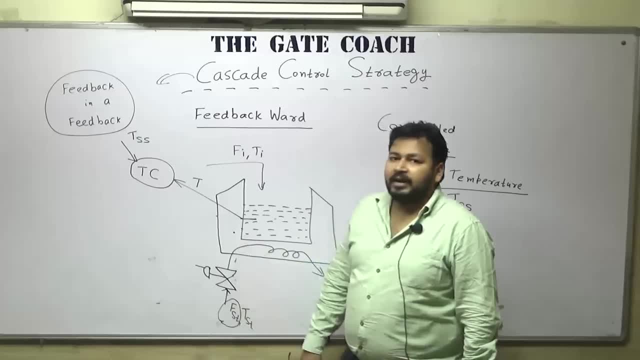 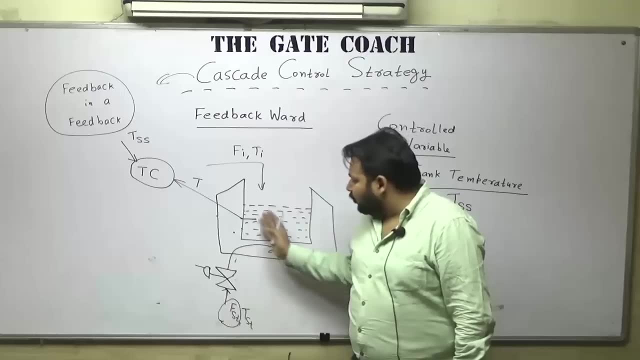 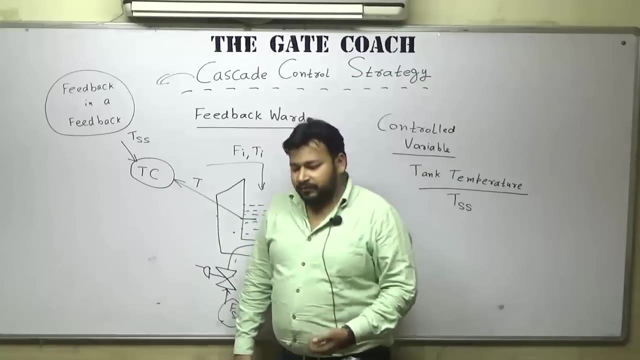 valve opening so that this flow rate can be achieved. so each things are interdependent. so what we need? we need a set of equations to solve this problem. this is the work of the temperature controller and to do this work it takes a lot of time, and that's why. 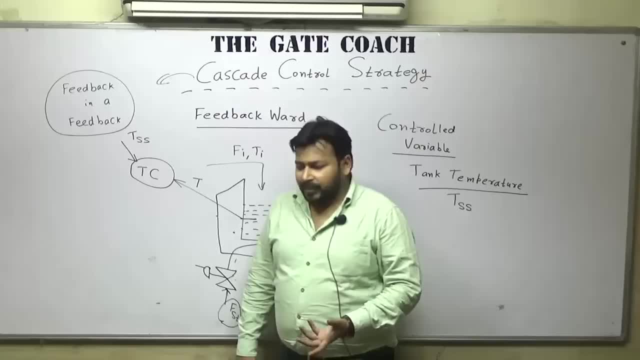 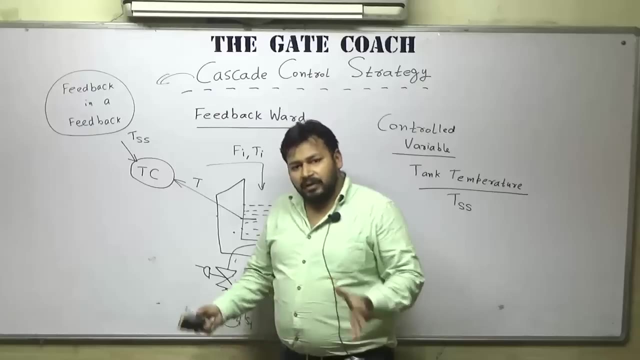 the feedback control strategy is slow or you can say sluggish, but in the case of cascade, what we do, we divide the work. that means in this case, now temperature controller is not the only one who need to do all the work. we will put one more controller that will help. 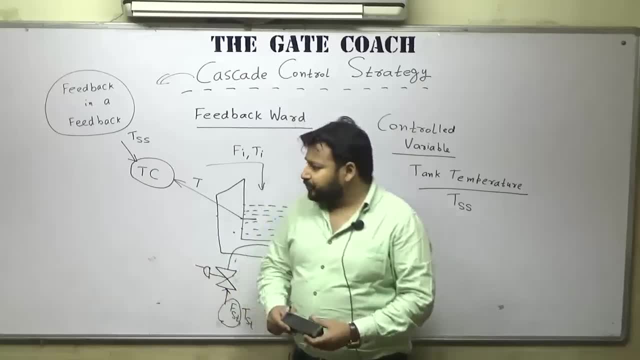 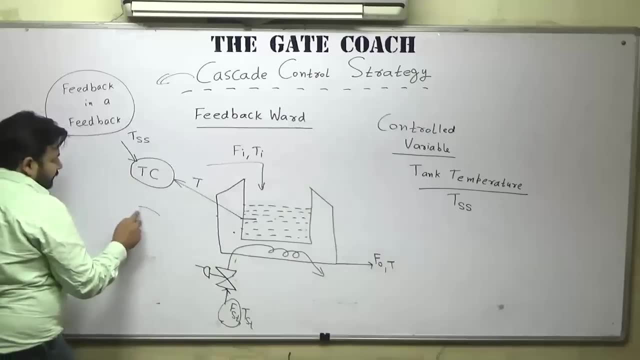 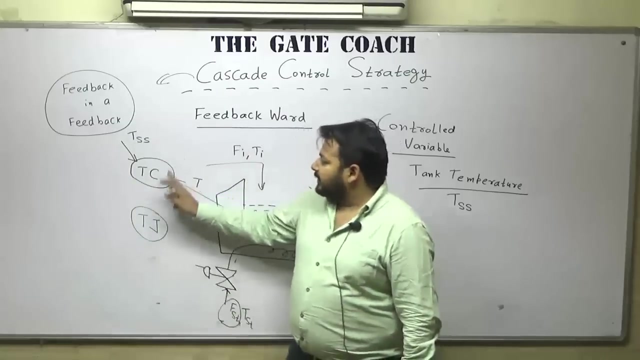 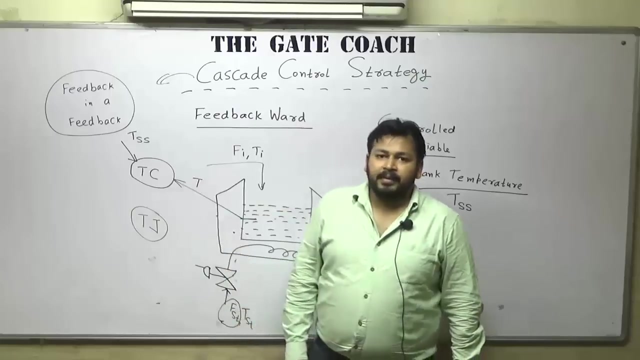 the temperature controller. to solve the problem Now with this controller, I will use another controller, and it's the jacket controller that will take care of the jacket temperature. so now, in this scenario, what is the work of temperature controller? the work is only and only to calculate the ideal jacket temperature. 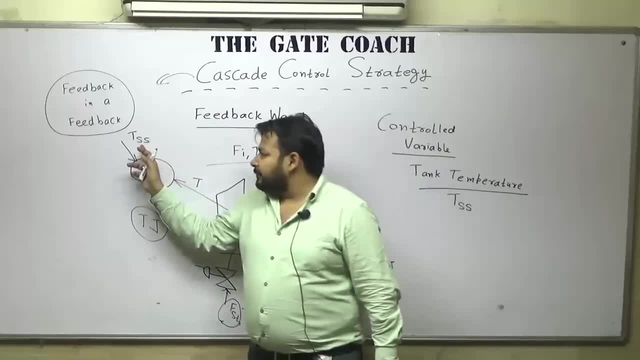 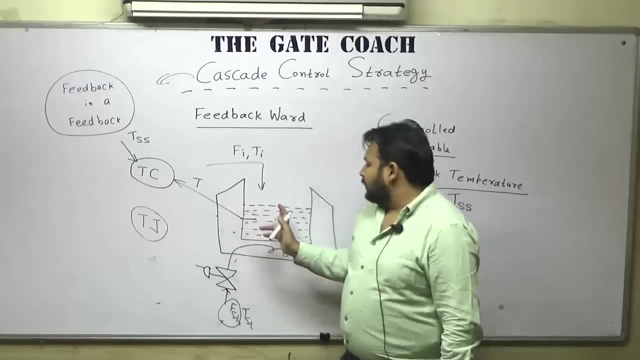 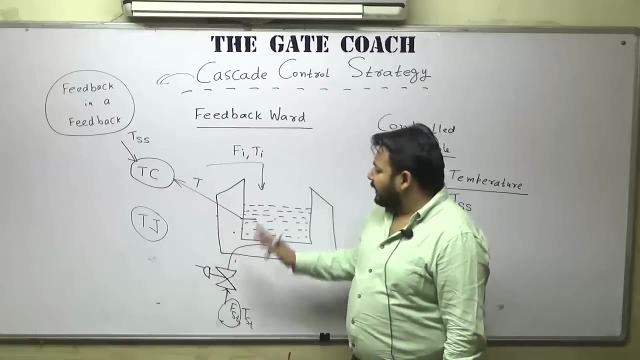 for example, Let's say the desired temperature is 50 and this temperature is also 50. the error is 0, this temperature is 50. that means, with respect to this temperature, there must be a jacket temperature also. and let's say, the ideal jacket temperature in this case is 52, because 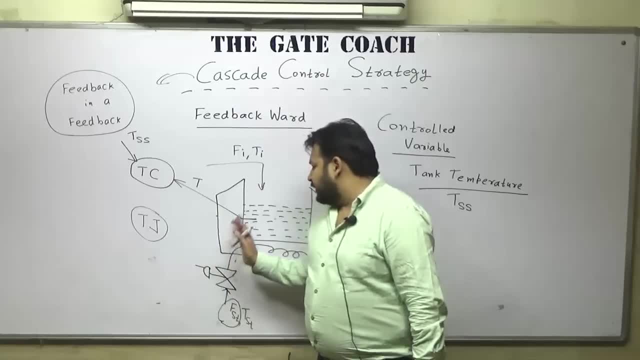 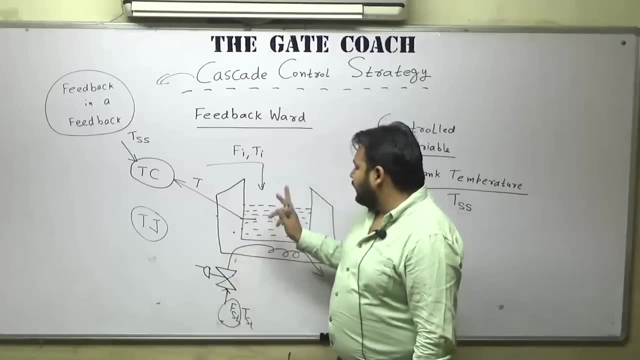 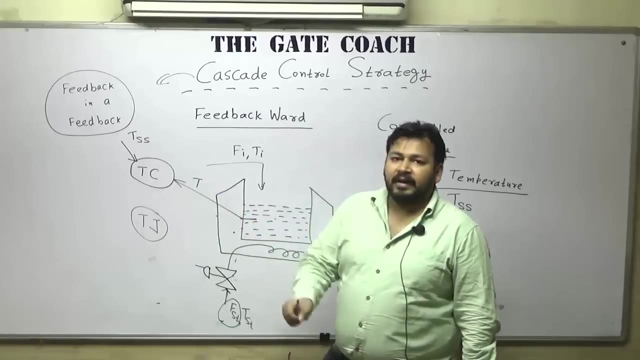 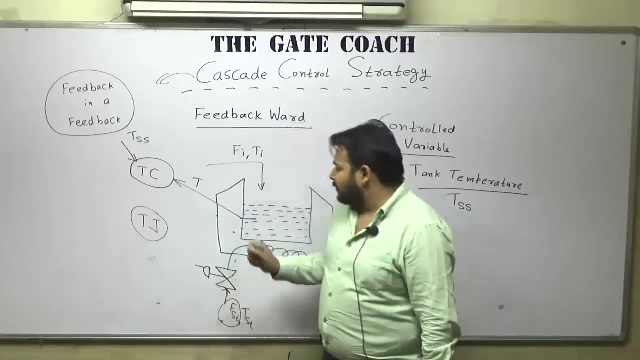 there will be some loss also. so, and this is 50 degree for the time being example. Now let's say this: 50 reduces to 48, so that means this is 50 and this is 48. there is an error. and to minimize that error, what will it do? it will calculate by what degree jacket temperature must. 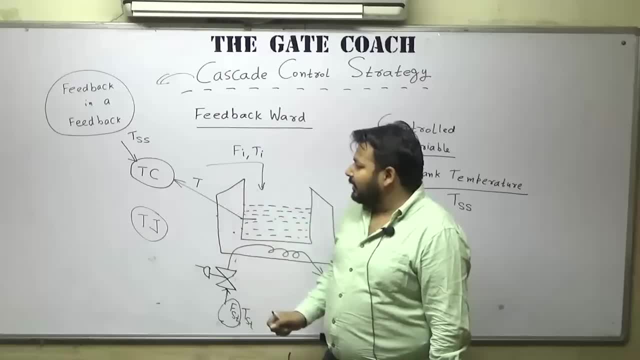 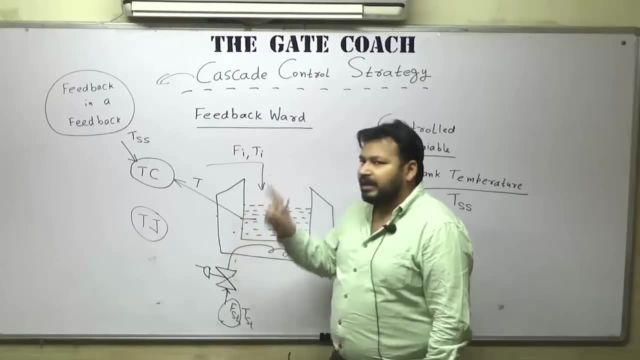 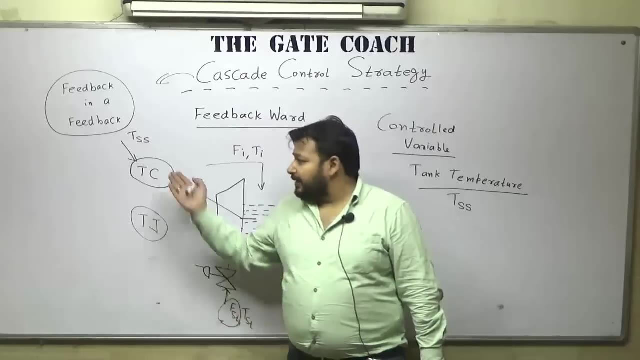 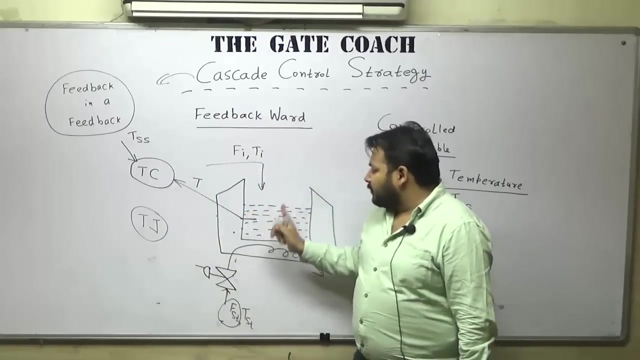 be raised. or in other words, it will calculate that to keep this 48 back to 50 again, what should be the ideal jacket temperature? Whether it be 53 or it is 54? that depends upon the equation. but what is the work? only one work: that to maintain the desired temperature in the tank. what should be the desired jacket? 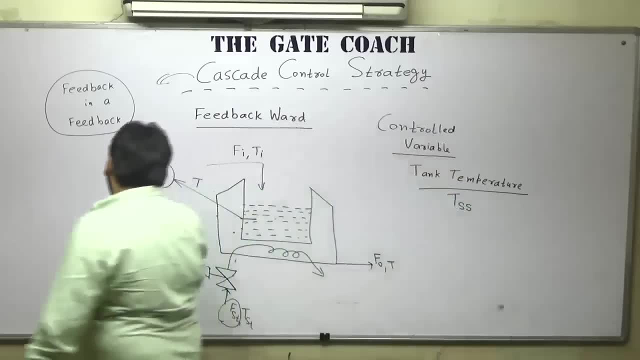 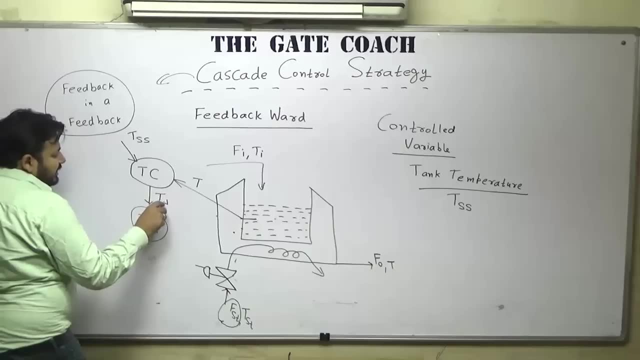 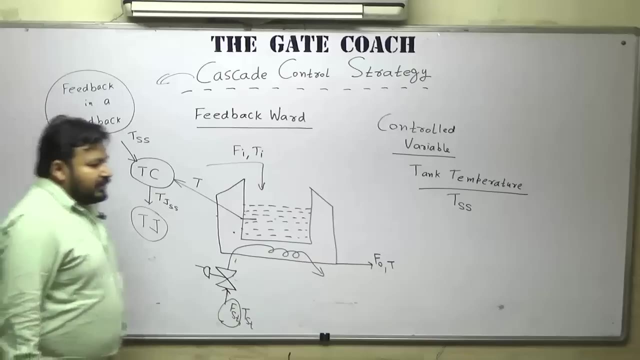 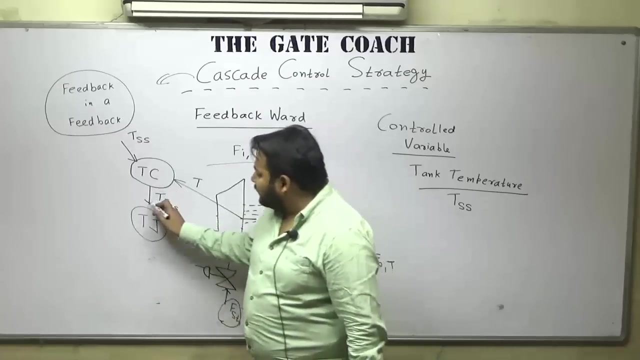 temperature. only one work. So, with the help of this error, what it calculate? it calculates that desired jacket temperature. Whenever I say desired, it means the steady state, desired jacket temperature. And after calculating this data, it will send this data to another controller, another controller. 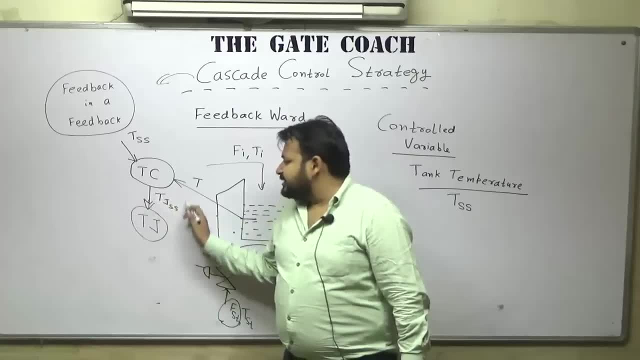 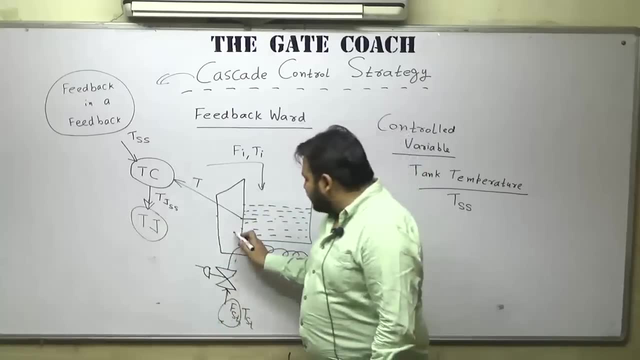 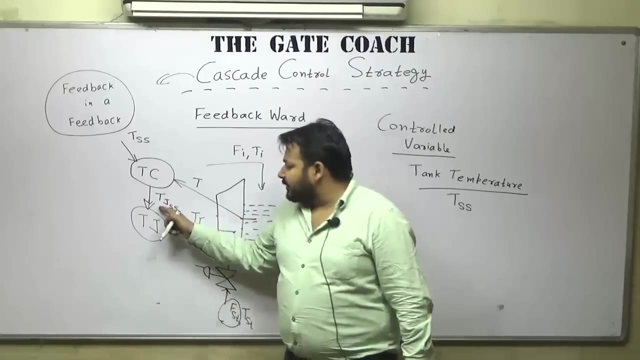 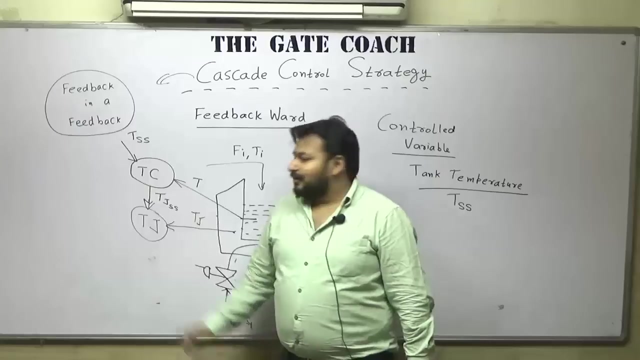 And now that means what should be the jacket temperature. Now, what is the jacket temperature? That jacket temperature is this: This is the actual jacket temperature, This is that jacket temperature, The actual jacket temperature, and if this, then it will do its own action. 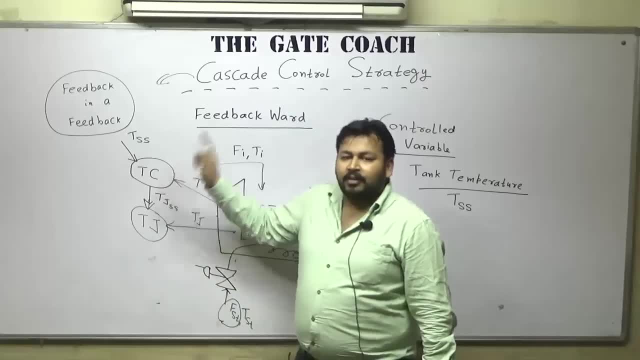 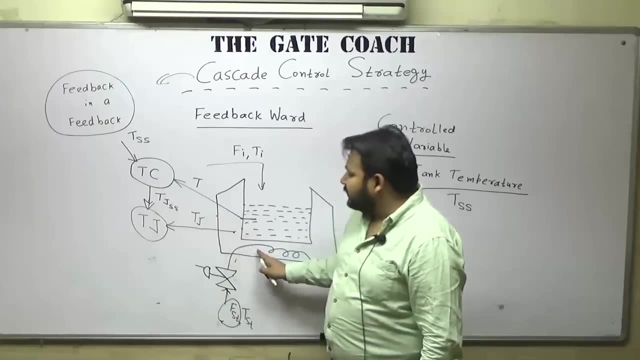 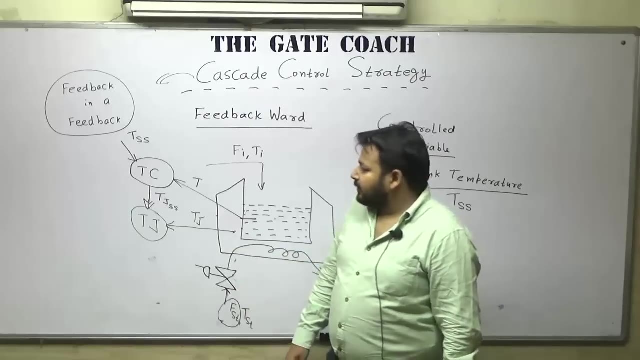 Now, what is the action here? One work is already done. What is the work left? The work left is to attain this ideal jacket temperature. what should be the steam flow rate? What should be the steam flow rate so that we can attain this temperature? 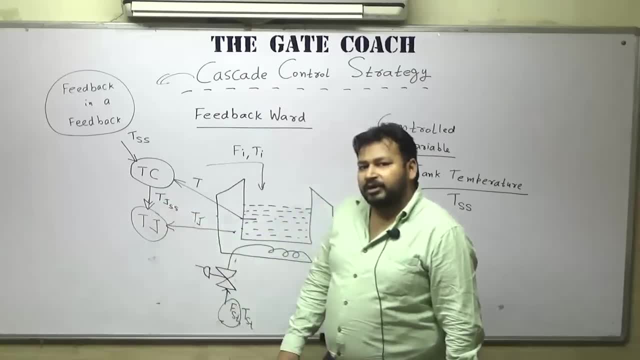 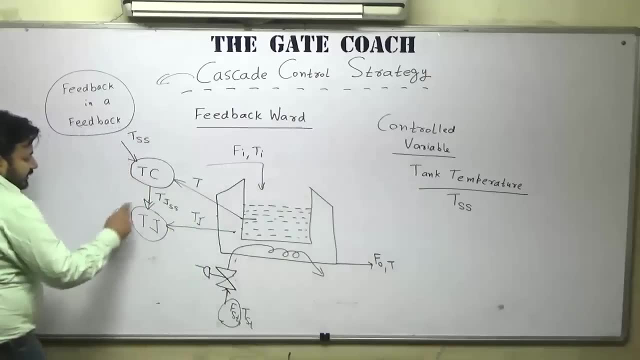 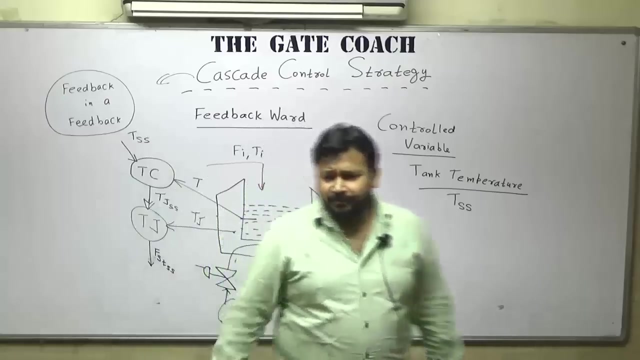 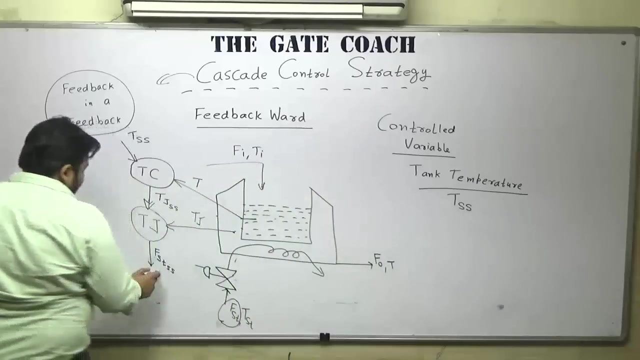 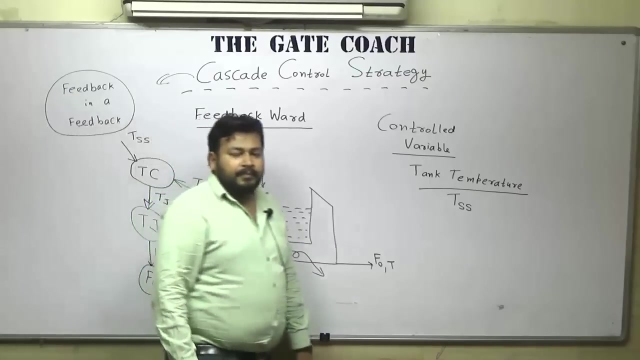 So to attain this TJSS, what should be the ideal steam flow rate. Now, this is the work of the jacket controller. it will calculate the best possible steam flow rate. Best possible steam flow rate. It is calculated, and now this data is sent to and the flow controller measures that. what? 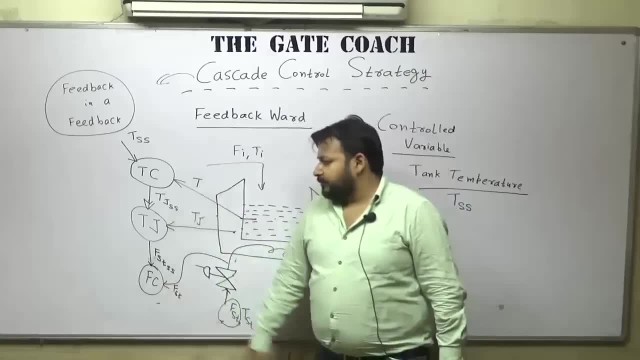 is the actual steam flow rate. It will calculate that Now. if there is any error, Then to calculate the actual steam flow rate. Now, if there is any error, Then to calculate the actual steam flow rate. Then to calculate the actual steam flow rate. 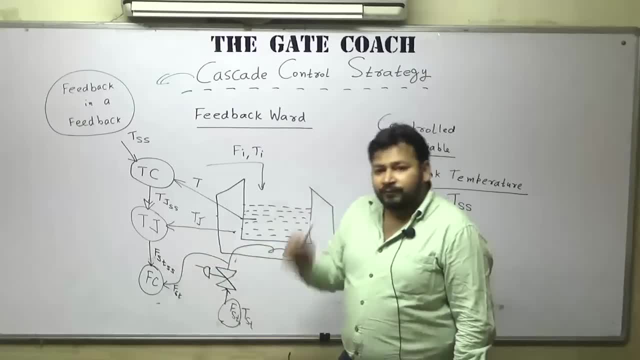 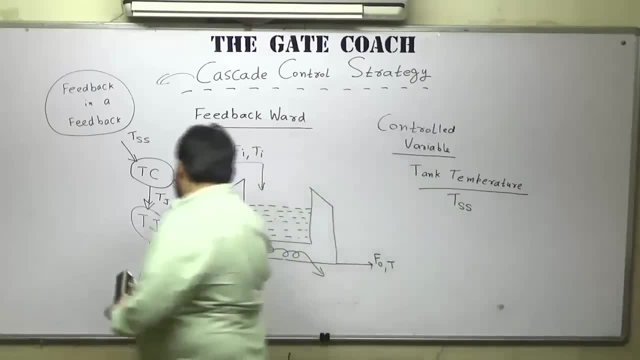 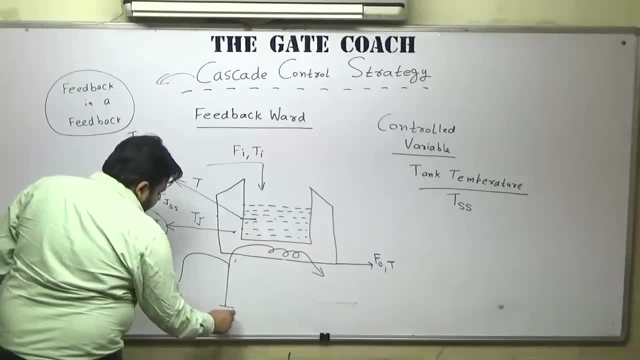 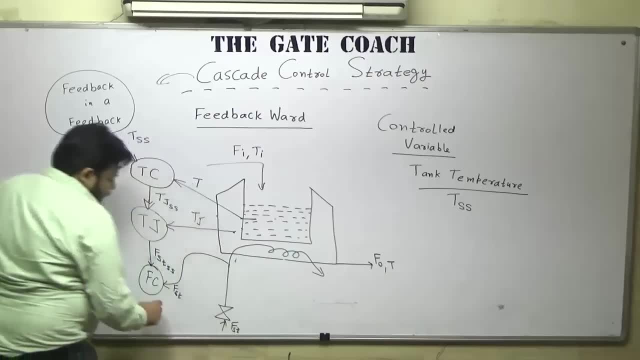 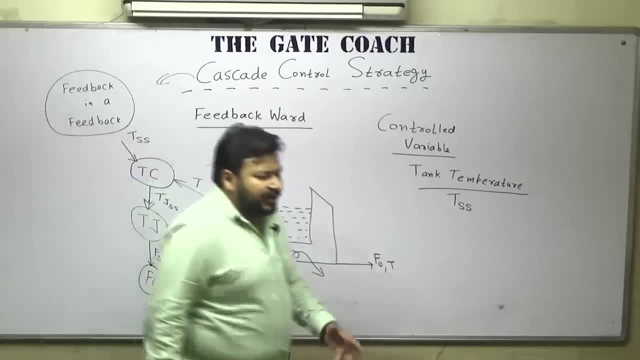 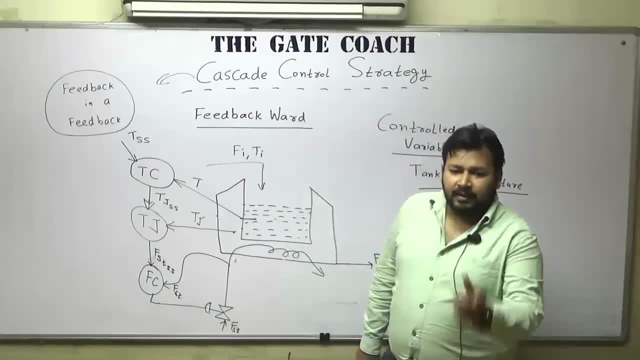 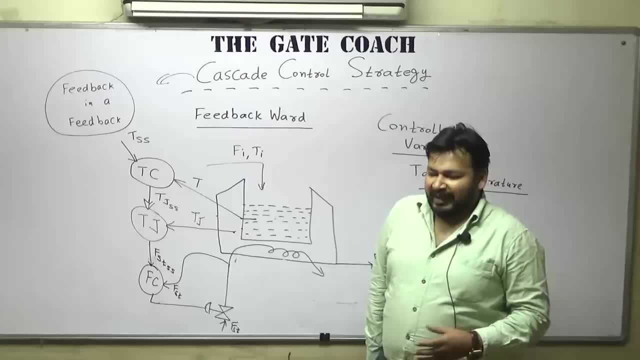 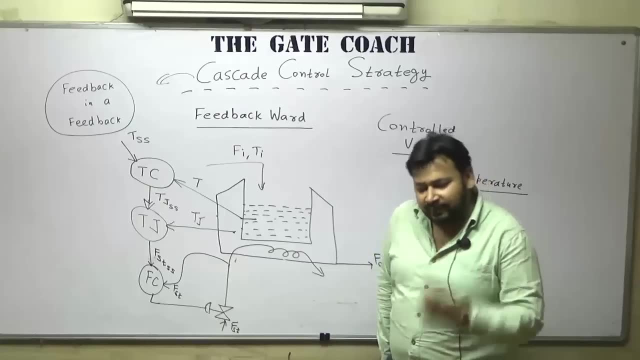 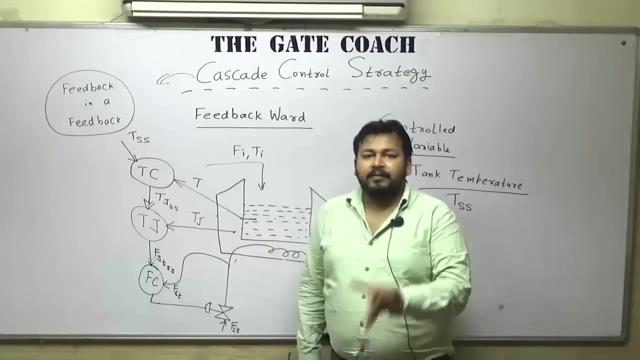 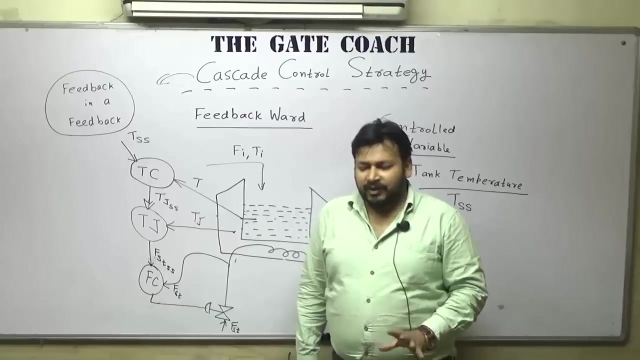 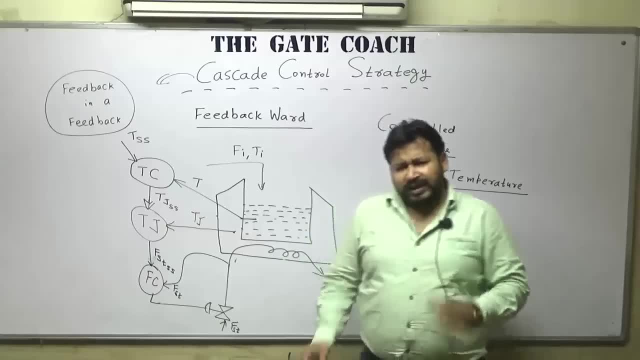 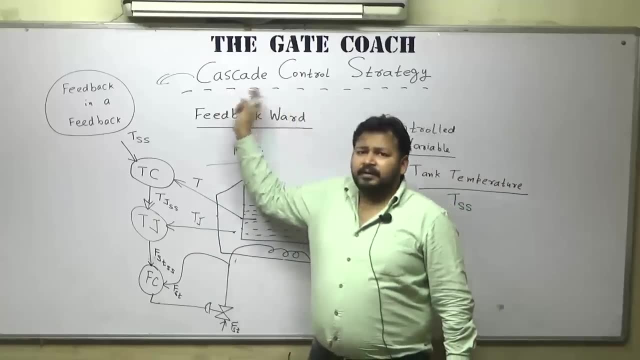 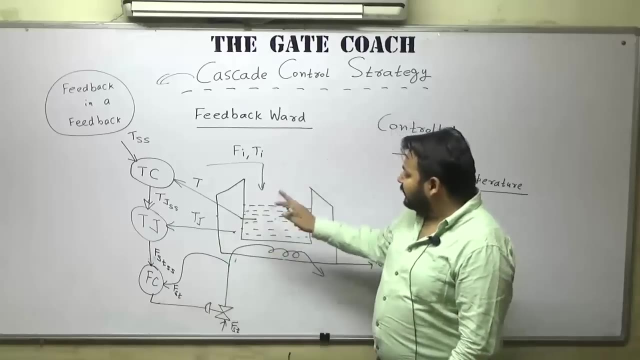 That is the only purpose. So cascade does that purpose. Feedback means one person is doing all the things. Cascade means there are more than one persons that is doing. those are doing the same thing. So what is that same thing? That same thing is to maintain the temperature of the tank. 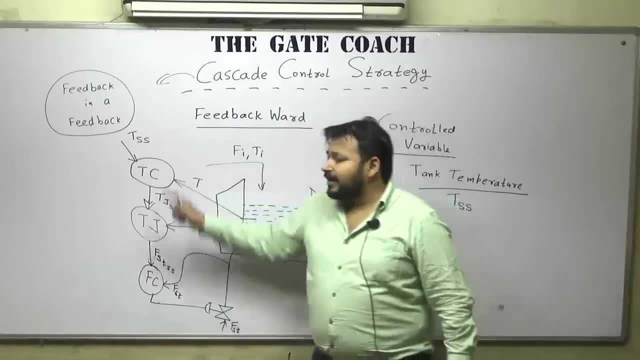 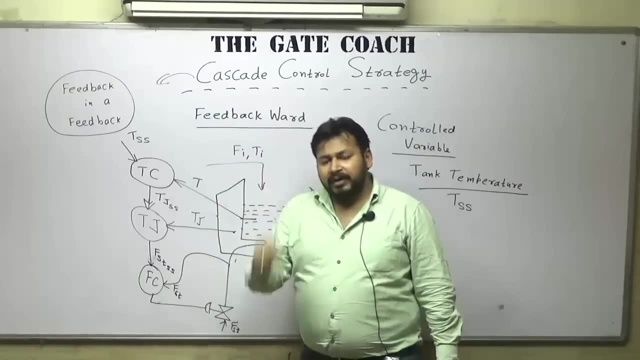 In the case of feed backward, that thing is done only by the temperature controller, But now, in the case of cascade, that thing is done not by one, Not Not by two, but by three controllers. So automatically the work will become fast. 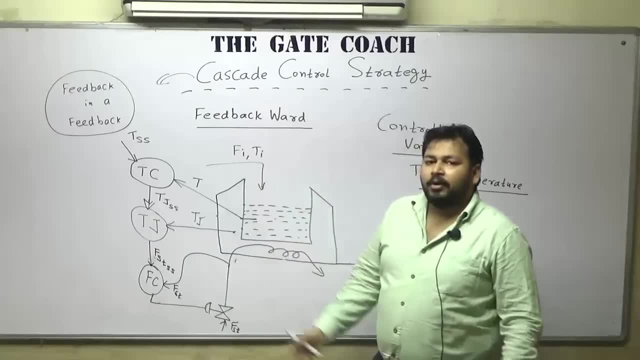 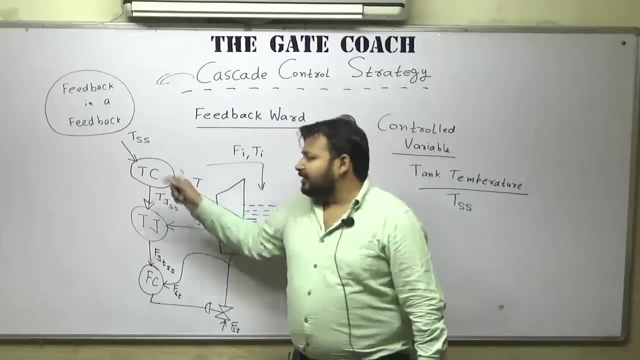 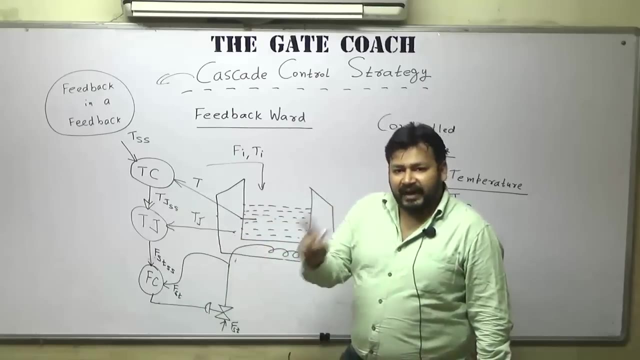 And now look at this: If there is any change in the FI, what will happen? This will change And this change is immediately sensed by the temperature controller. If there is any change in the jacket temperature, then that change is immediately sensed by the jacket sensor. 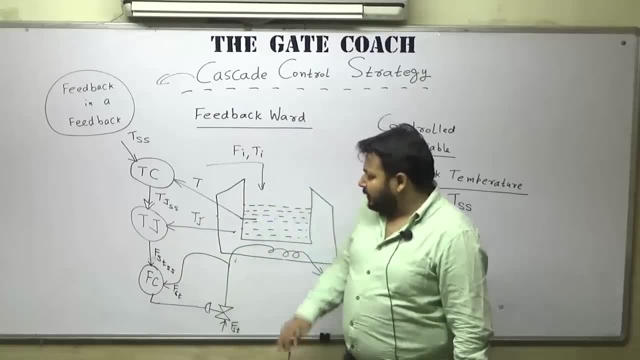 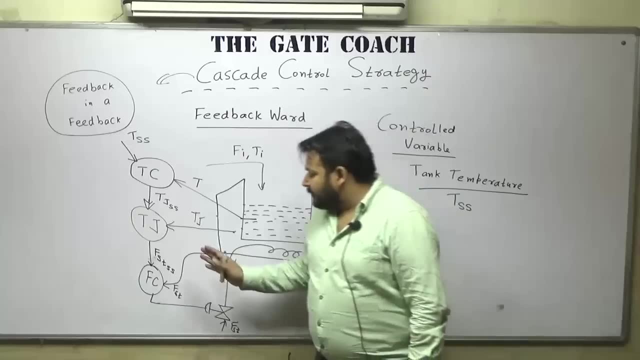 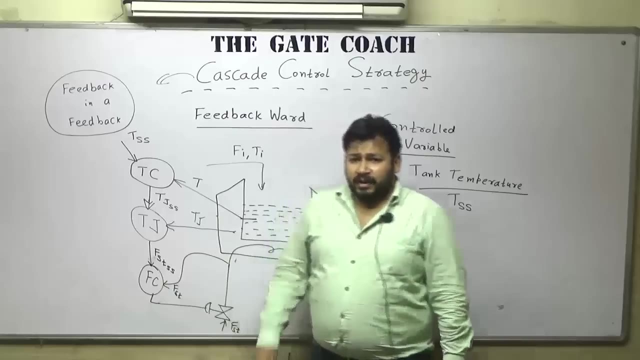 And acted upon by the jacket controller. If there is any change in the steam flow rate, then that change is immediately sensed by the flow sensor And acted upon by the flow controller. That means now this strategy is effective not only for the one, not for the two, but for the three disturbances. 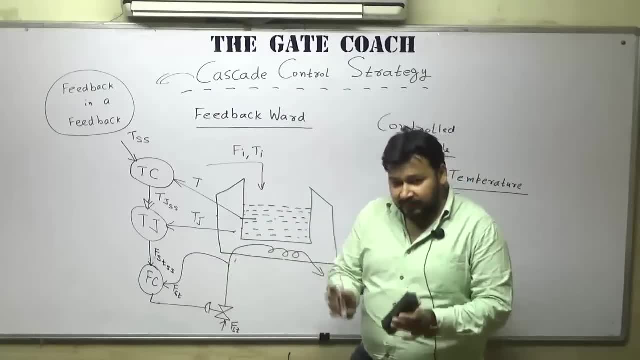 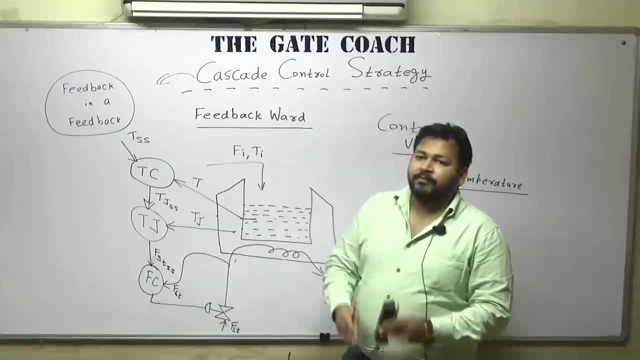 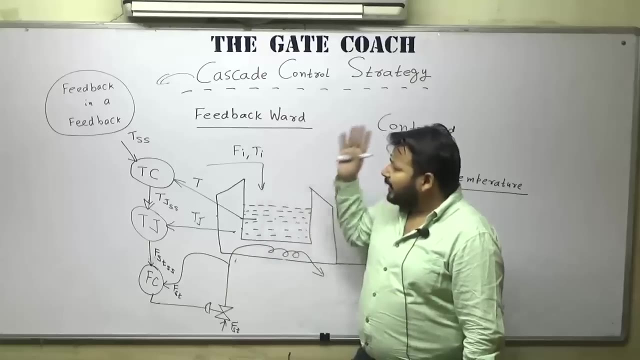 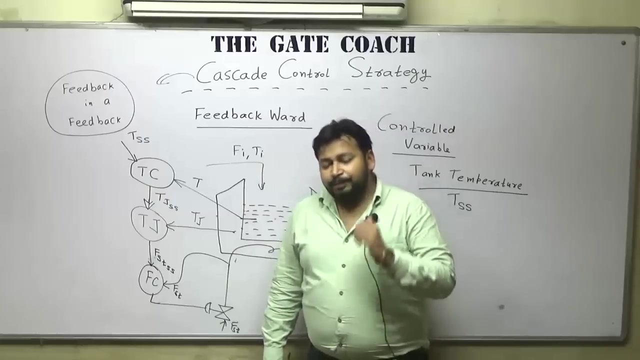 It remains fully effective, fully awake, fully switched on. That is, if there is any type of change, any type of disturbance, any type of non-ideality in the system, the controllers are there to act upon it. And that is the advantage of the cascade control strategy: that it gives us the advanced control. it gives us better control as compared to the feedback control strategy. 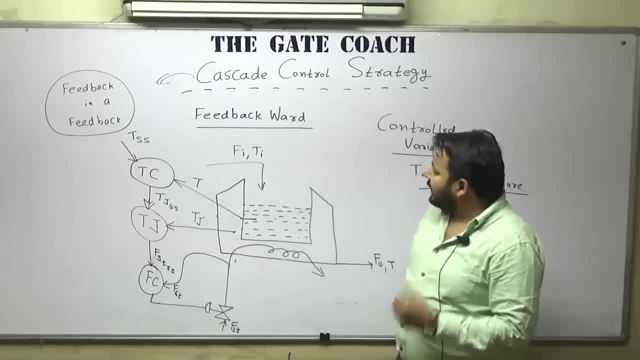 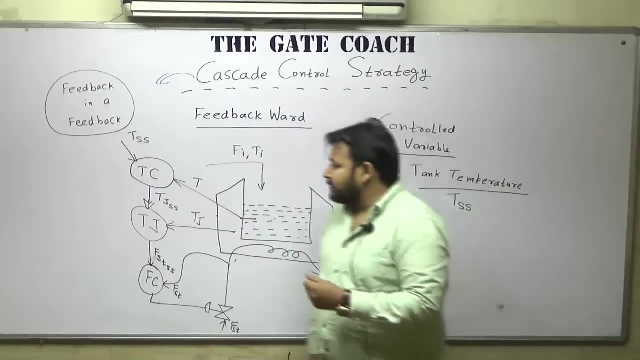 Okay, So this is all about the cascade control strategy. Now I will tell you about the cascade control strategy. So this is all about the cascade control strategy. Now I will help you to name some of the things here, those which help you in the interview as well as in the gate preparation also. 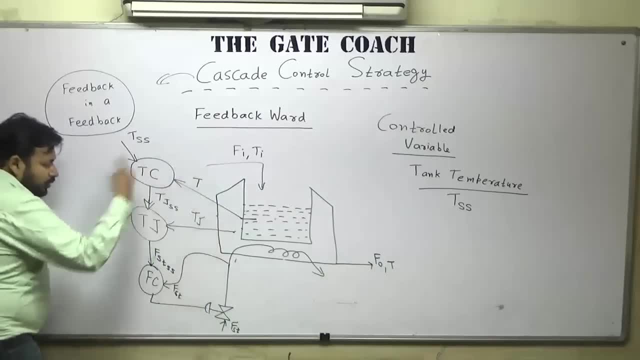 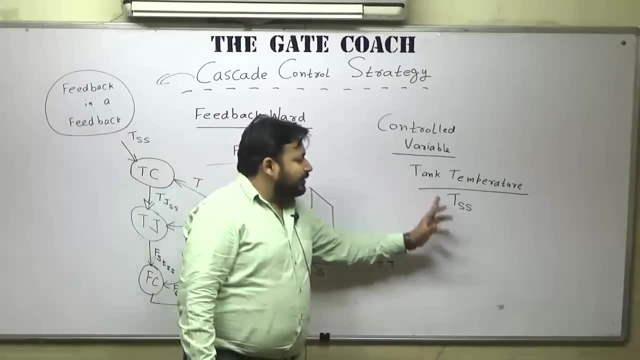 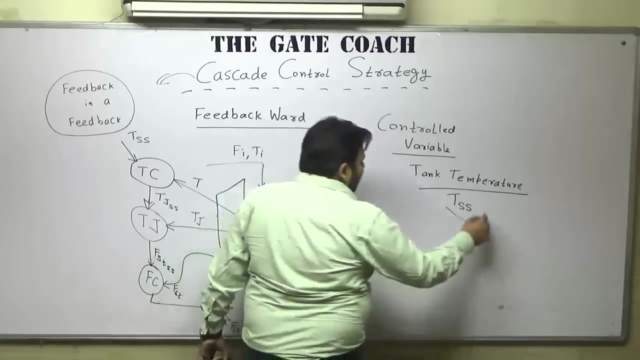 Now in whole, in the whole system, in the whole strategy, what is our main purpose? Our main purpose is to maintain the temperature of the tank. That is our main purpose. So whatever is the main purpose, that main thing becomes the primary. 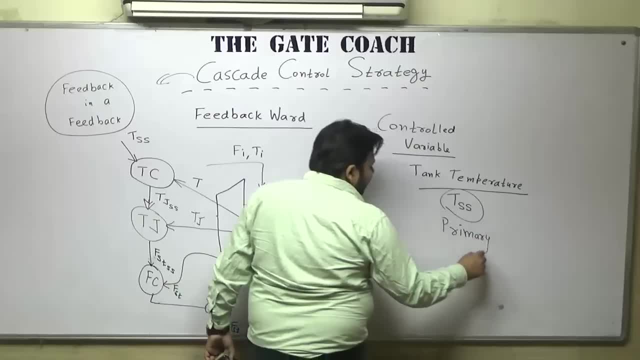 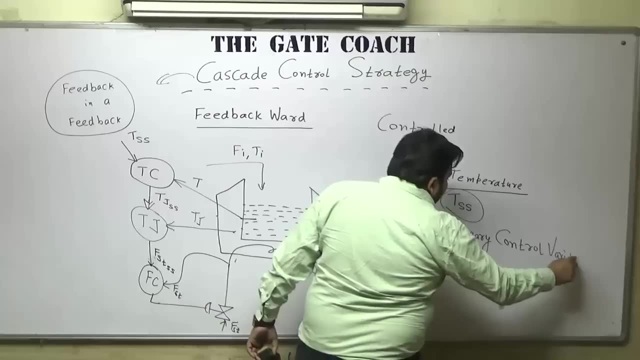 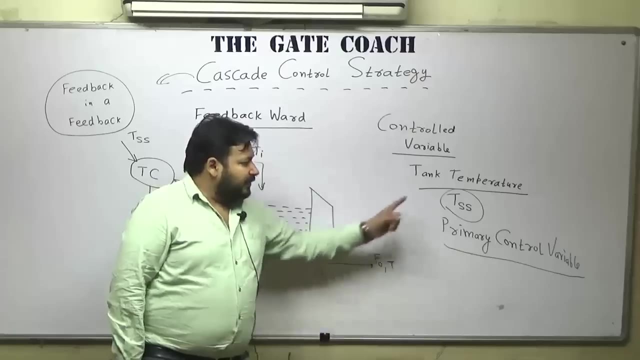 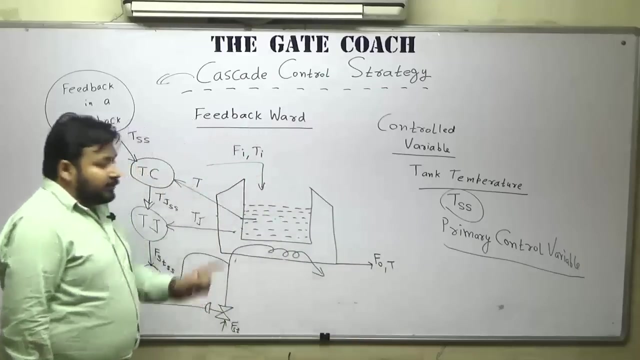 So this is primary variable, or you can say the primary control variable. It is not only the control variable, it is the primary control variable. So what is primary control variable? The variable that is to be maintained by us. And in the whole strategy, you can see, there is only one input: that is given by us, that is given by the user, that is given by the engineer. 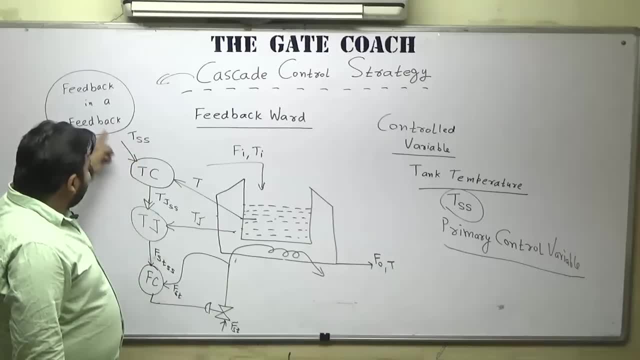 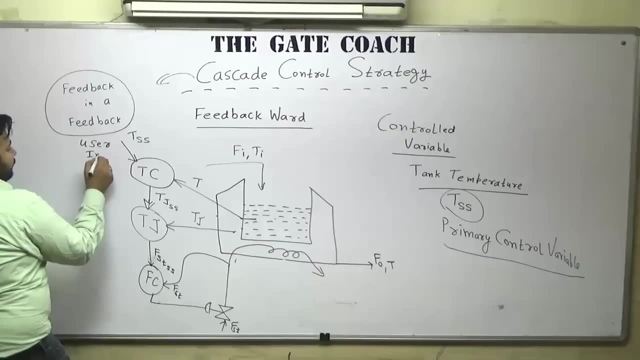 And that is this. You can see the source. What is the source? It is the user input. That means we will put that It is the user's input. So whatever is the user input, that user input becomes the primary control variable. 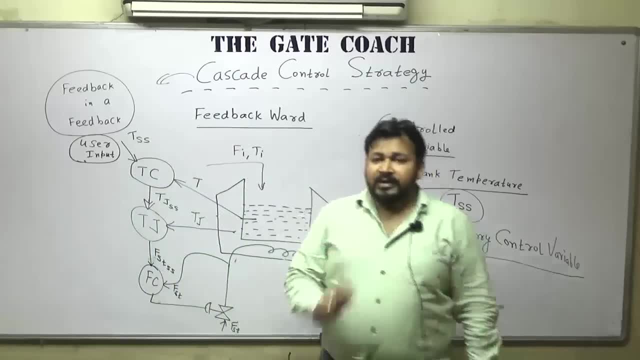 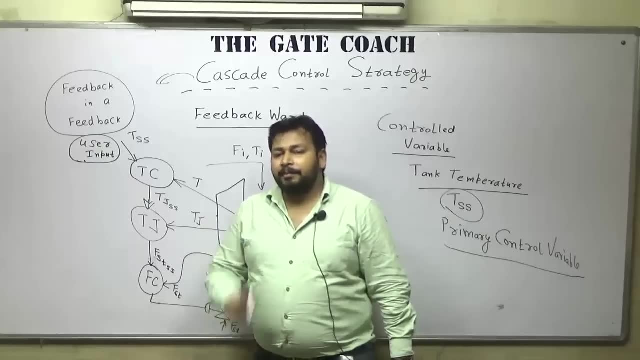 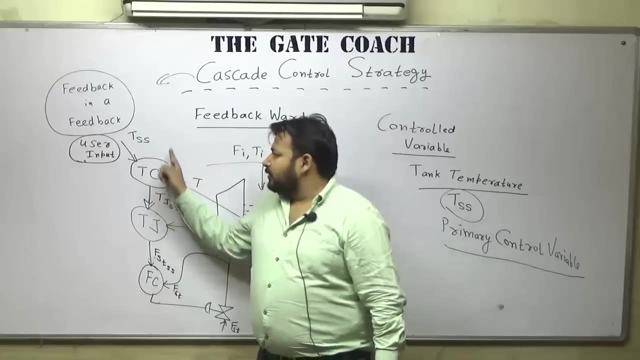 I hope you can understand it Now. whatever is the controller that helps us to serve, the primary control variable becomes our primary controller. So, out of these three controllers, this TC helps us to fulfill this value, to attain this value, to achieve this value. 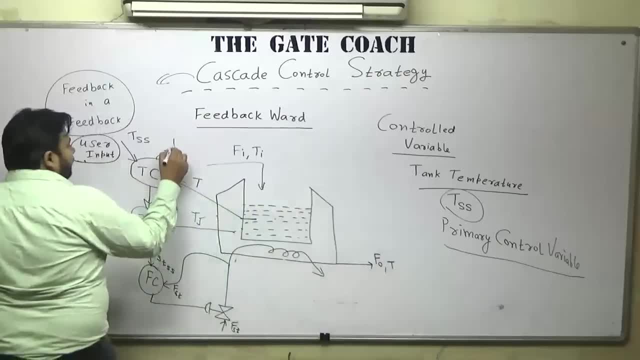 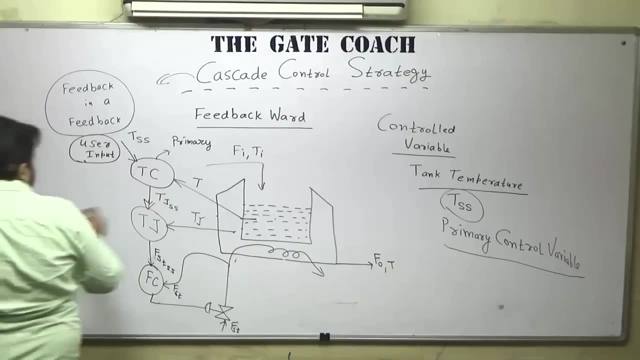 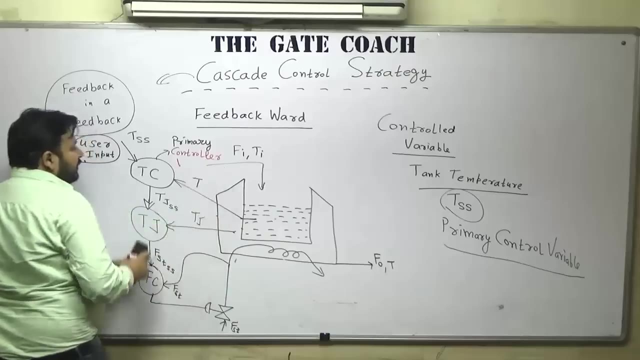 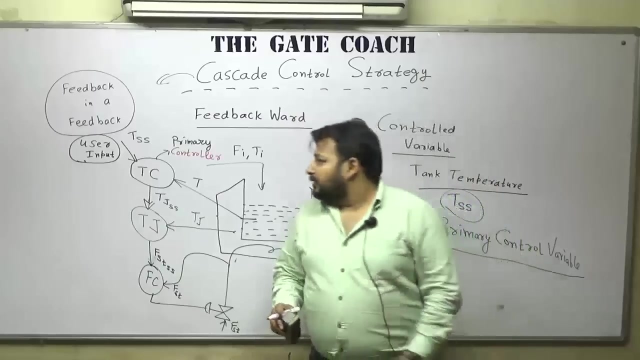 That is why this controller becomes the primary control variable. I will write it with another marker, So primary control variable, Primary control, Not variable. It is the primary controller. The controller that achieves that, helps to maintain the user input value, the primary control value. that becomes the primary controller. 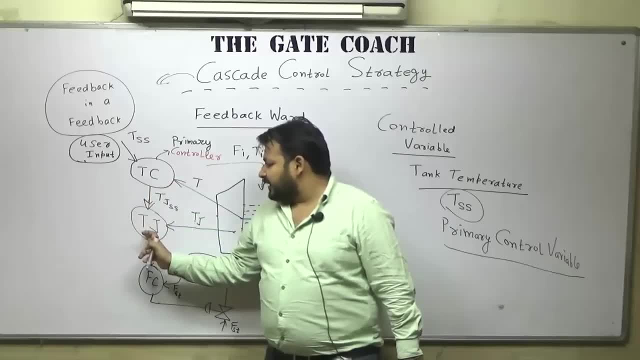 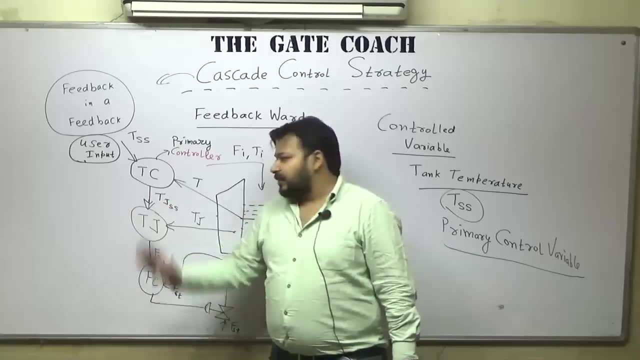 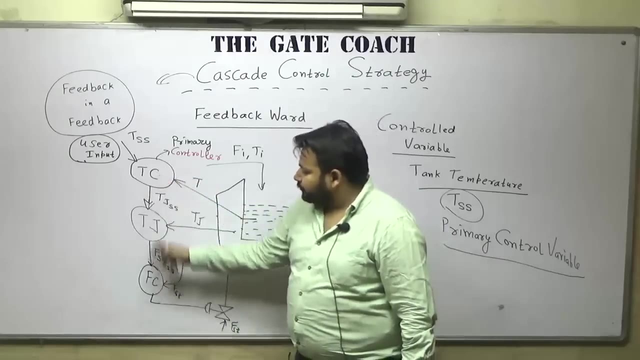 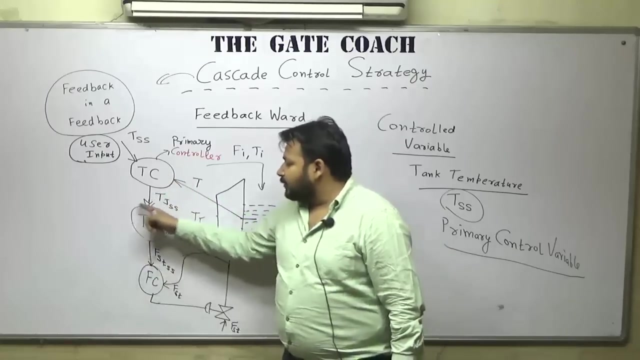 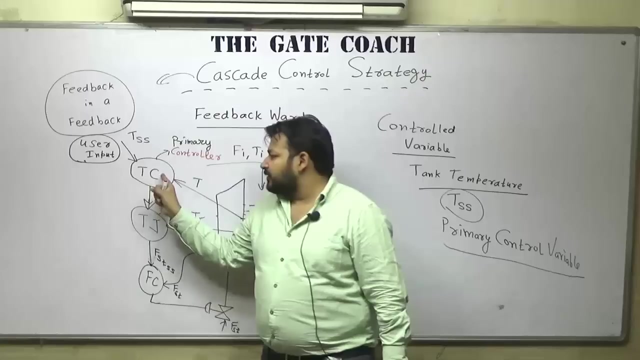 Now, if this is primary, this becomes secondary and this becomes tertiary. If there is fourth one, then again, then fifth, then sixth, but this remains the primary controller And it is giving the Signal to the owner. That means for this controller to work, it needs a signal from this controller. 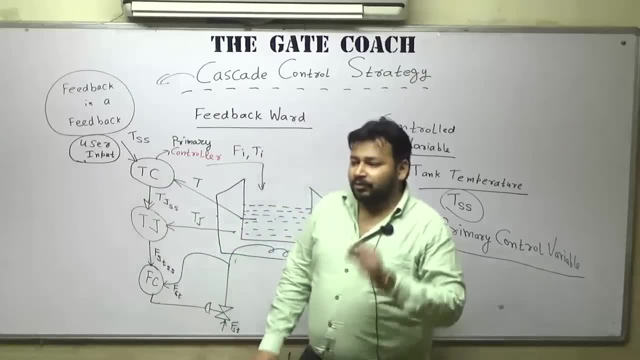 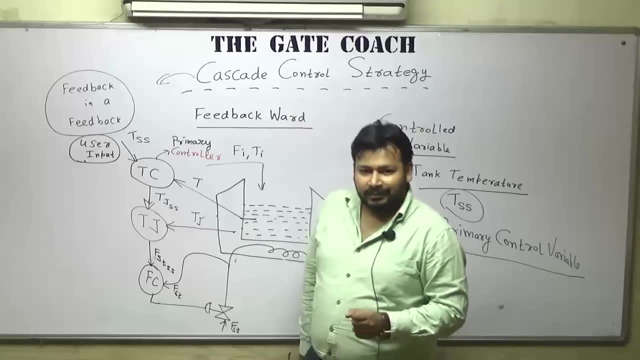 That means like in an organization: without the order of the boss, an employee cannot do the things on its own. It needs an order. In an army, it needs an order of a general What to do, And then the army man will do that thing. 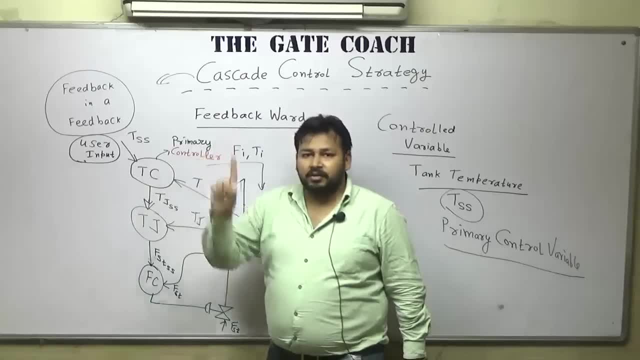 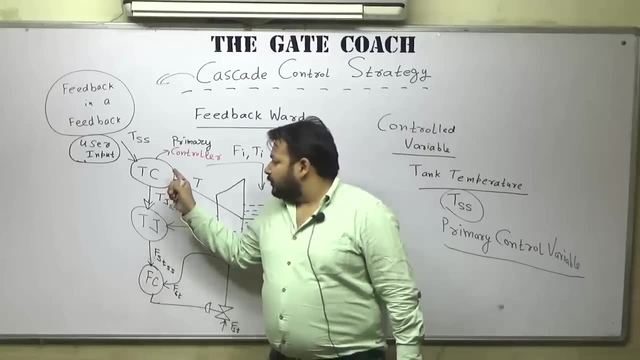 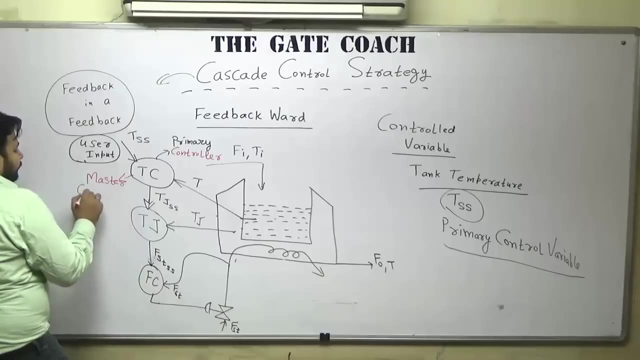 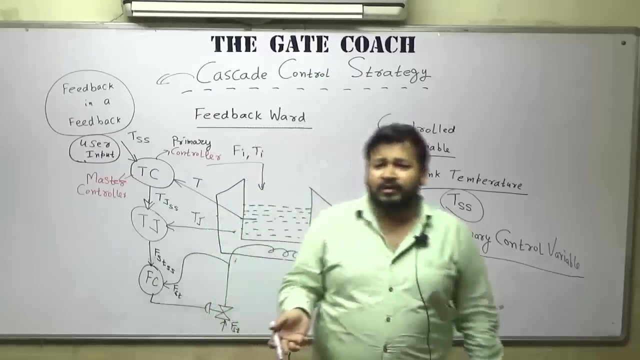 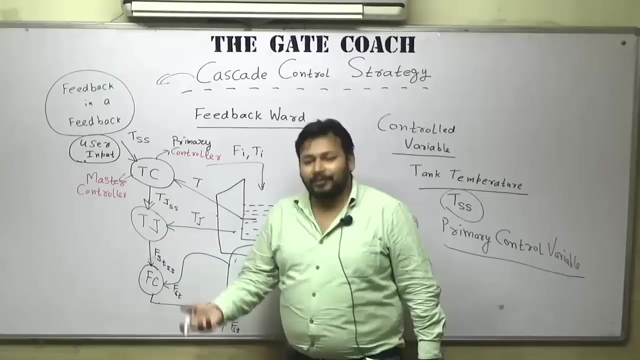 So here this becomes the master controller, Because it masters the complete loop, It owns the complete loop. So this also is known as the master controller. And then the rest of the controllers becomes what? Employee controller? No, They becomes the slave controllers. 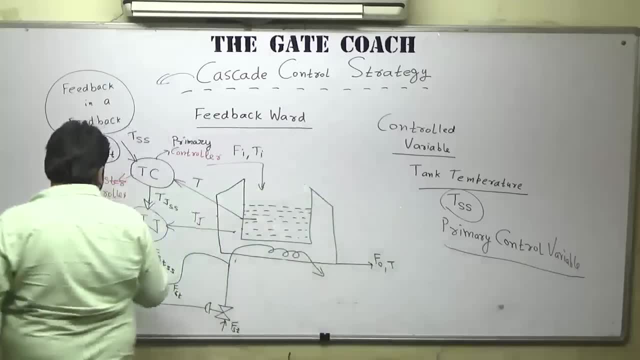 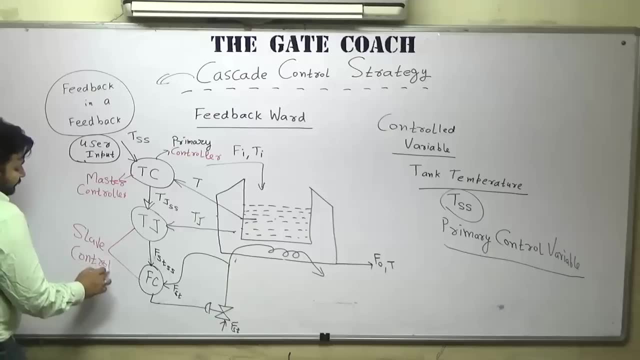 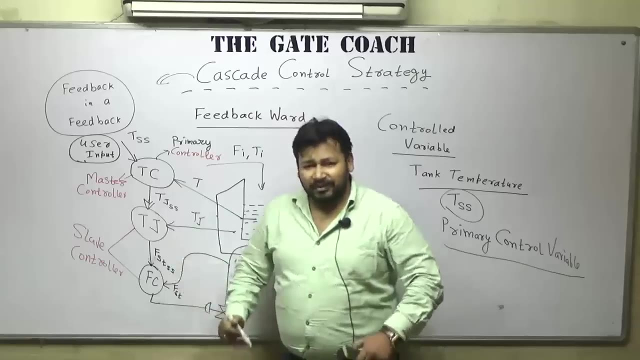 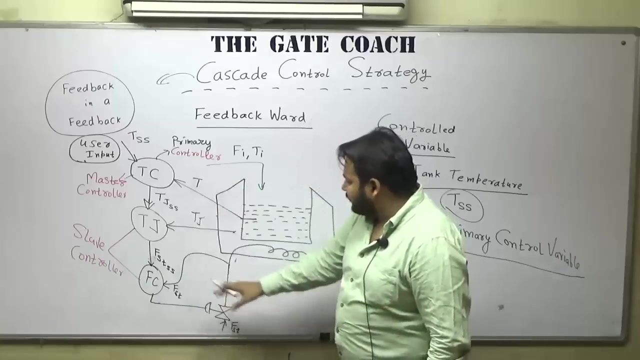 The more worst word. Note the employee controllers, synonym of the employment. So this is master controller, the bossy controller, and this is slave controller, Some kind of employee controller. So this is the scenario, This is primary control variable. 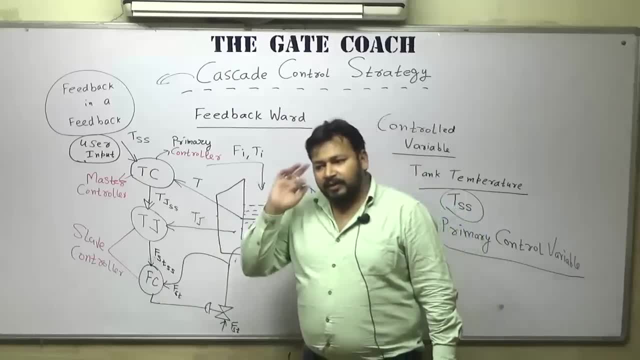 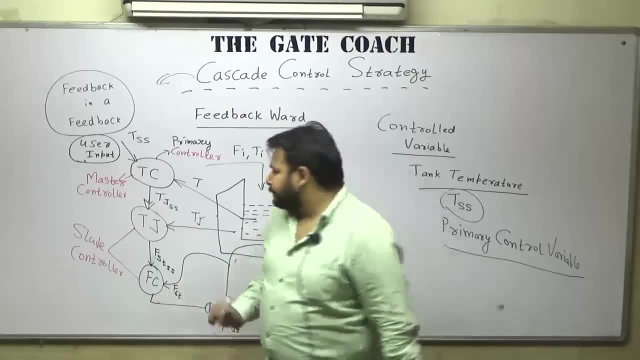 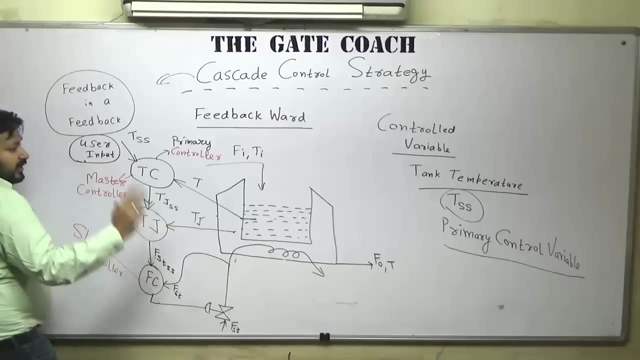 The whole strategy is cascade. Now, how you will identify cascade? Cascade is nothing but the feedback, Any feedback. Or you can see that one measurement, two measurement, three measurement, There are three measurements, But look at the manipulated.